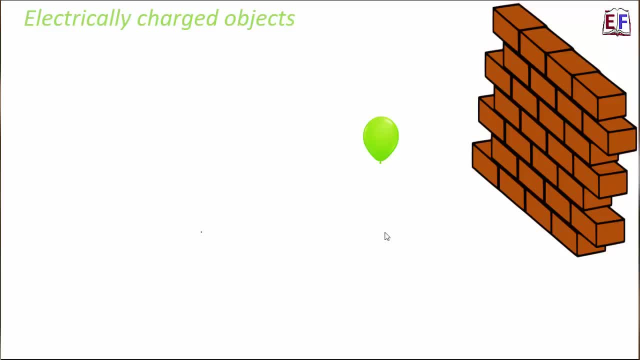 you bring this balloon near a wall. Do you think that you will be able to stick the balloon to the wall without using fevicol adhesive or any cello tape? Of course not. But now you take the same balloon and rub it on a towel for some time, And after that you take. 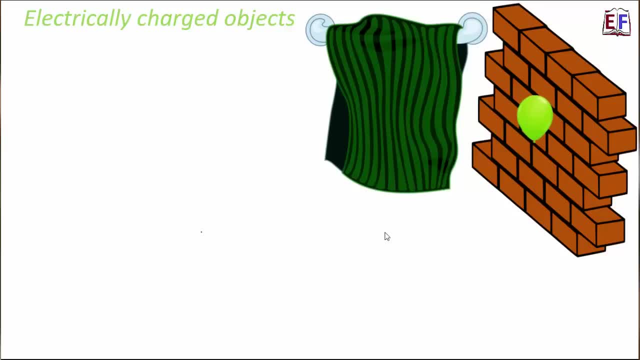 the same balloon near the wall and it sticks to the wall. What is this? Is this a magick? Not really. The balloon gets electrically charged by rubbing with the towel. Let's look at another example. These are some bits of paper. You take a plastic comb. 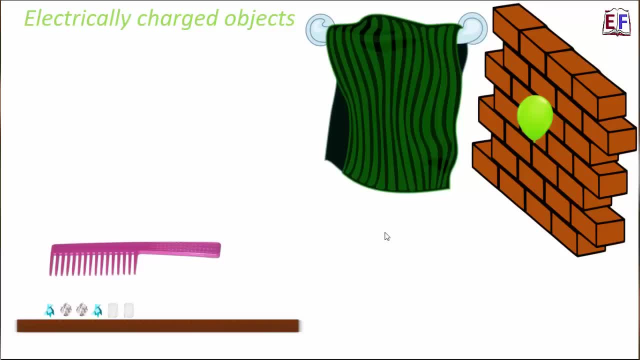 bring it near these bits of paper. What happens? Nothing. Now you take the same comb and comb your hair for some time. After that you repeat the same thing. bring the comb near the bits of paper. time you see that the bits of paper are dancing. that's because they get attracted towards the comb. 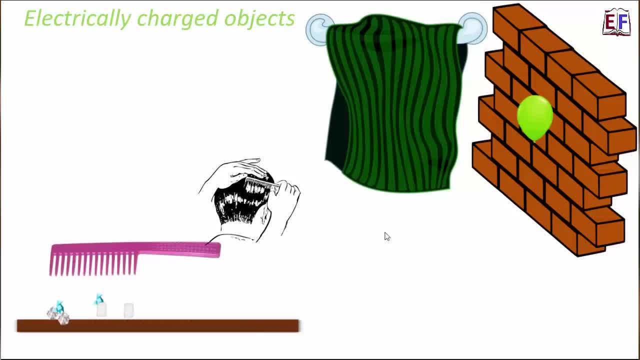 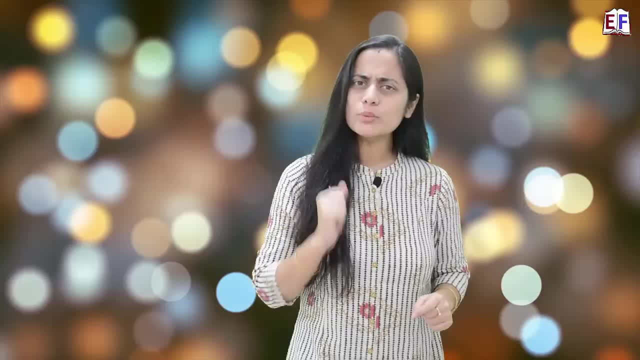 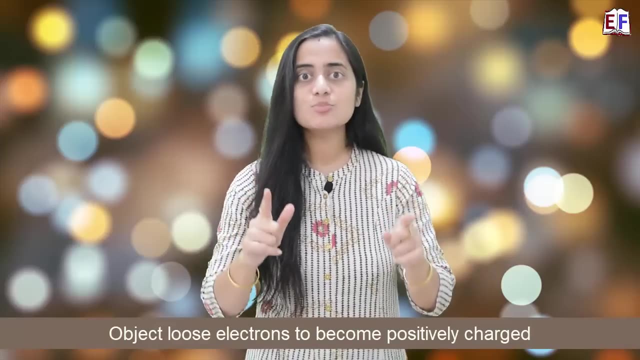 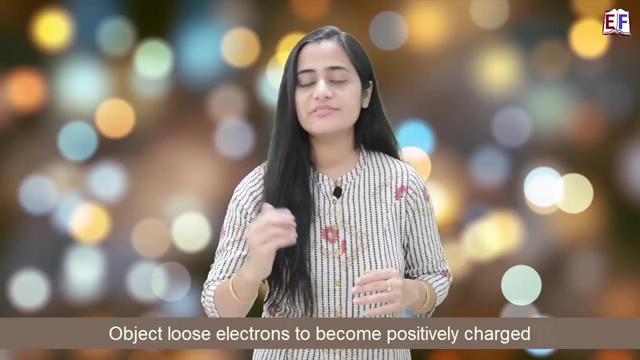 why? because the comb here is electrically charged by rubbing with your hair. electrically charged could be positively charged or negatively charged. now, what do we mean by positively charged? now, when an object has excess of positive charges, it is positively charged. that's quite obvious, right? so therefore, an object loses electrons to become positively charged in a similar way. 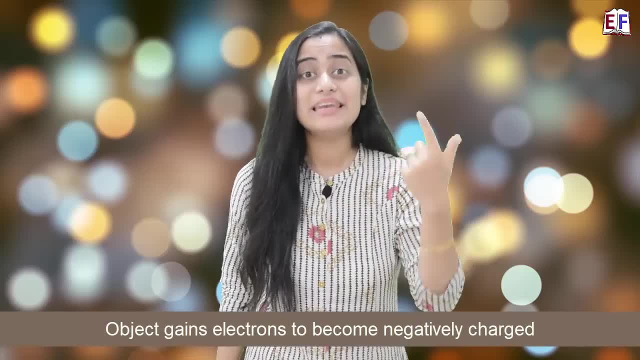 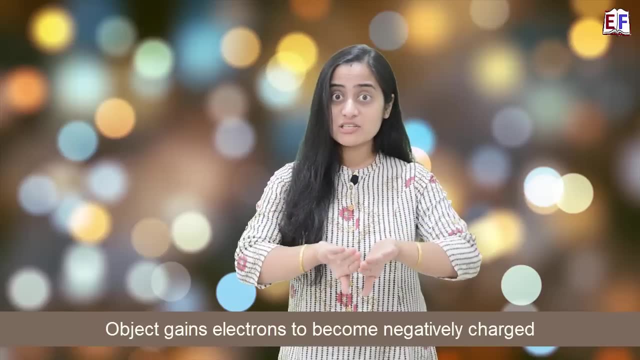 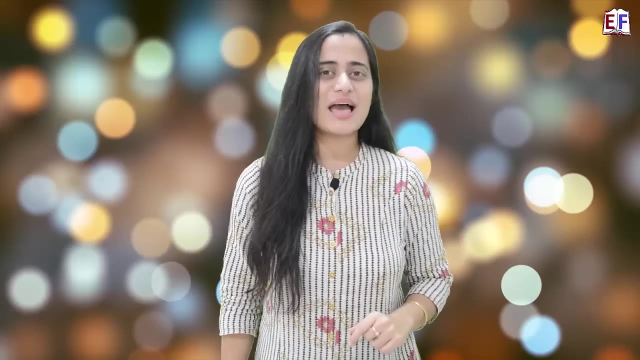 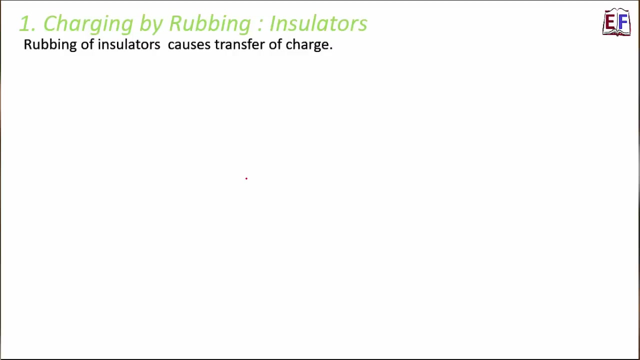 an object gains electrons to become negatively charged. now we also know that, like charges repel, as in positive, positive repulsion, negative, negative repulsion, whereas the unlike charges attract, so positive, negative attract. there are many different ways by which objects can be charged. the first method that we are going to discuss is rubbing, so charging by rubbing works. 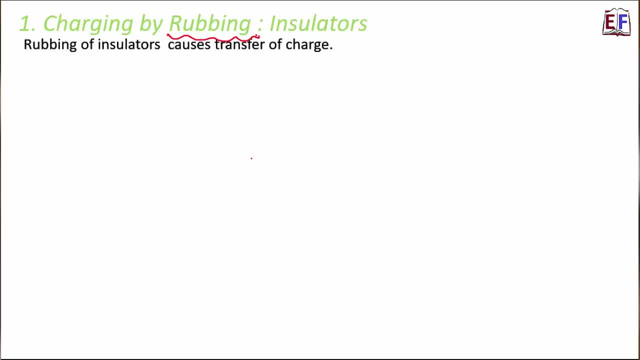 for insulators, that is, those objects which doesn't allow electricity to pass through them. now how? let's take a look. so here we'll again take the example of the comb, which got electrically charged just by rubbing with the hair. now that means in this case, transfer of charge took place. 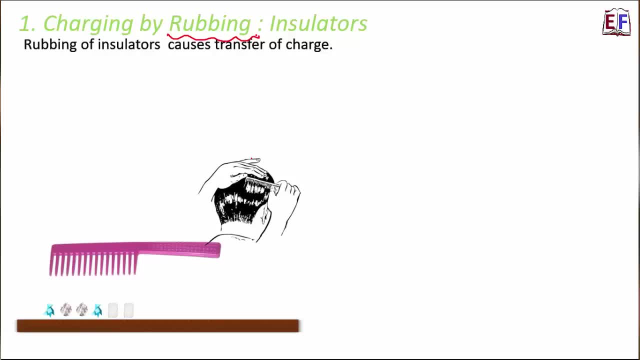 but the question is: how did the transfer of charge take place? as in the, the electrons move from hair to the comb, or from the comb to the hair. who loses electrons, who gains electron, and what decides that? that is where triboelectric series comes into picture. now, this series is as you can see. it is a. 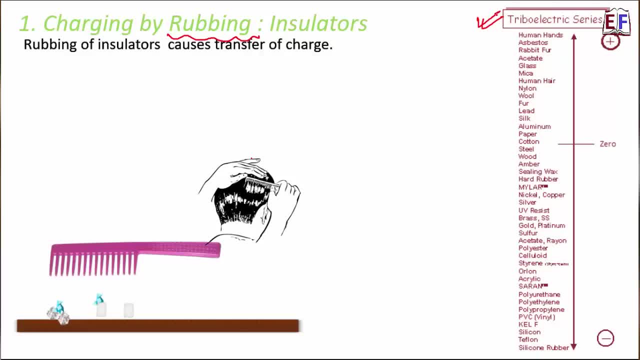 list of things which tells us that which of these objects have a tendency to lose electrons and become positively charged, and which of these objects have a tendency to gain electrons and become negatively charged. in fact, if you look at this list, all those things which are towards the 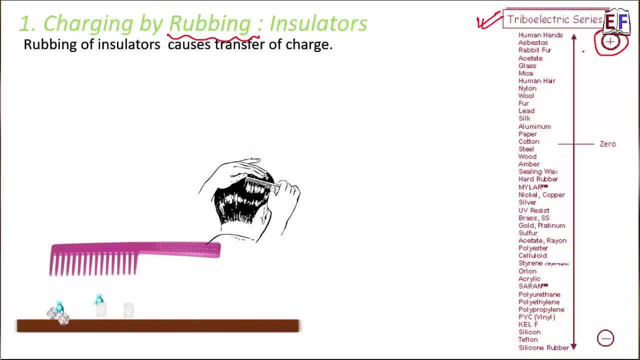 top, they all tend to lose electrons and become positively charged. and those towards the bottom are the ones which tend to gain electrons to become negatively charged, and those which are kind of at the middle are kind of neutral. for example, paper, cotton, steel, wood, they are kind of neutral right. so now, in this particular scenario, we are rubbing two objects. one is: 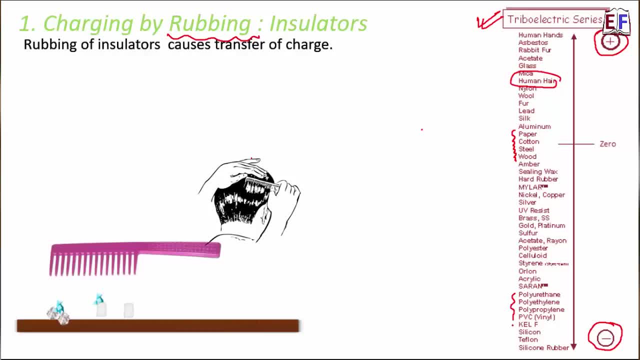 human hair and plastic, which is here right. so, as a result, we see that human hair is on the top side of the series, whereas plastic is towards the bottom. that means the transfer of electrons will take place from human hair to the comb, so the comb will gain electrons and, as a result, 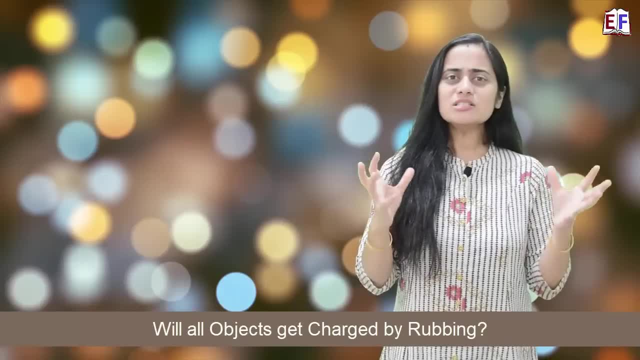 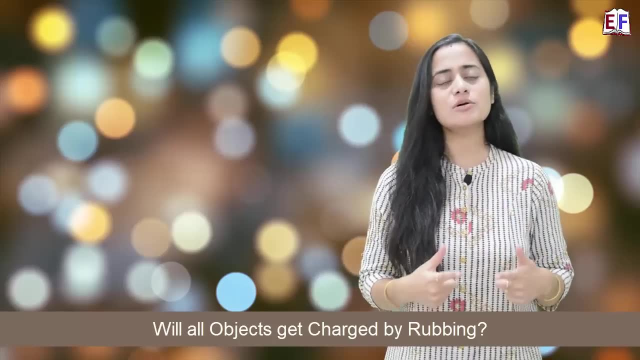 of this, the transfer of electrons will take place from the comb to the hair and, as a result of this result, the comb will become negatively charged. The process of charging by rubbing happens only for few specific pairs of materials. Do you know why? Because in this process of rubbing, very limited number of electron transfer happens. because 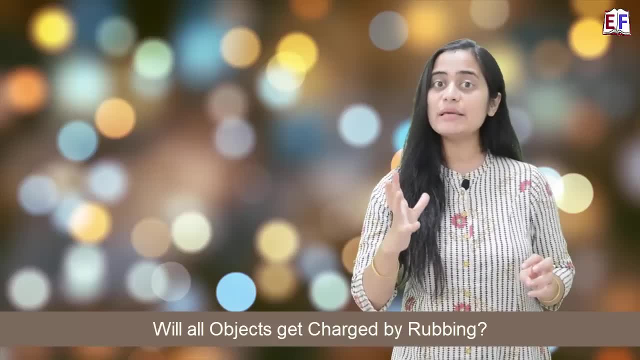 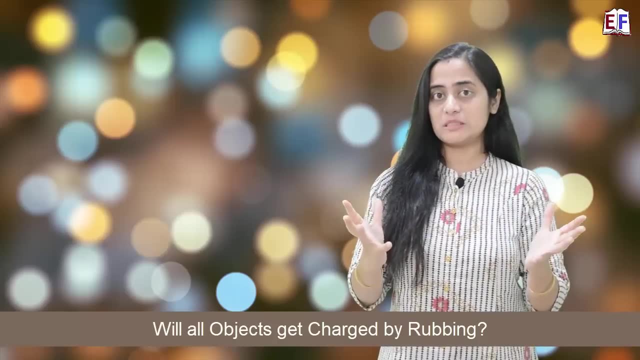 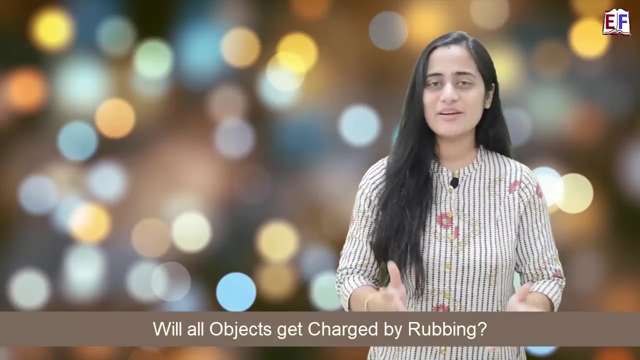 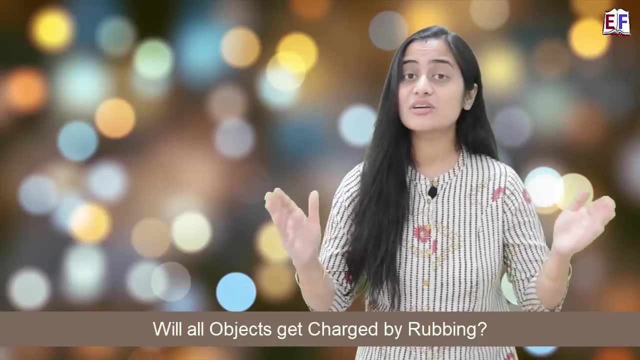 only those electrons get transferred which are less tightly bound to the nucleus. So therefore, we need an electronic configuration that should support this. Therefore, only those elements which have that suitable electronic configuration will be charged by rubbing. The very important point: charging by rubbing doesn't happen in case of conductors. 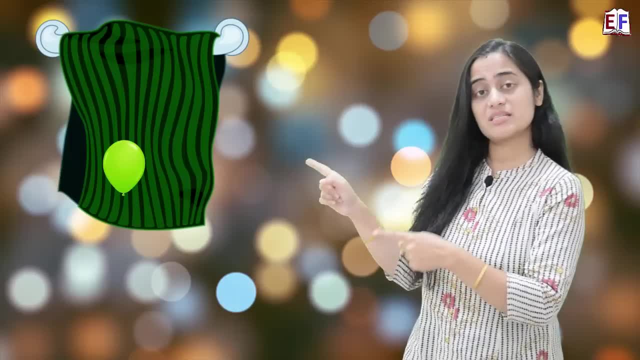 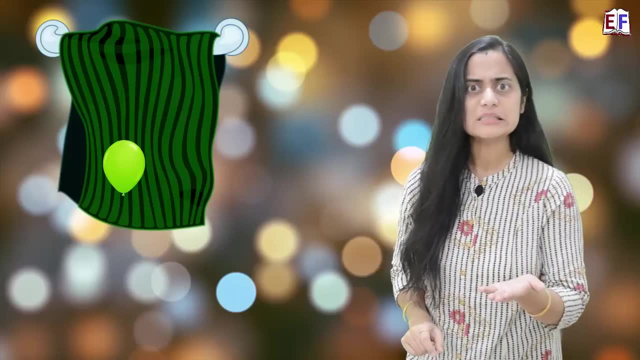 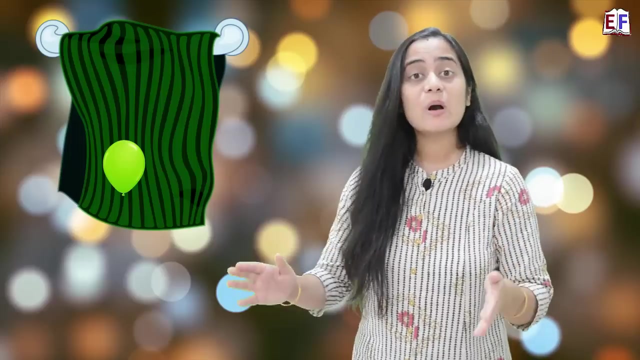 Try it out for yourself. If you repeat the same experiment that we did a little earlier, just replace the balloon with a metal key- What happens? No matter how many times you rub that key on the towel, it never sticks. Why? Because this is made up of metal, the key is a metal, and metal is a good conductor of. 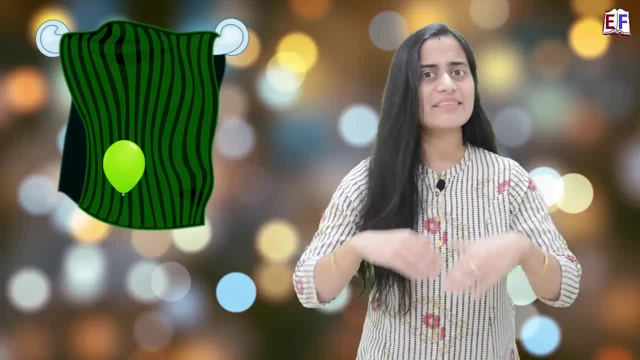 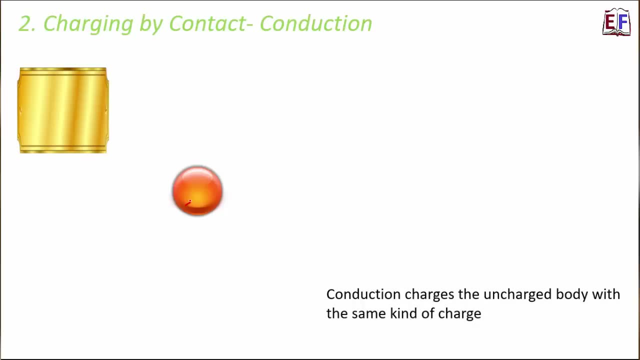 electricity and therefore it conducts all the charges and there are no charges on the surface of the metal. The second method of charging is by contact or conduction. Now, what happens in this is when an uncharged substance is brought in contact with a charged 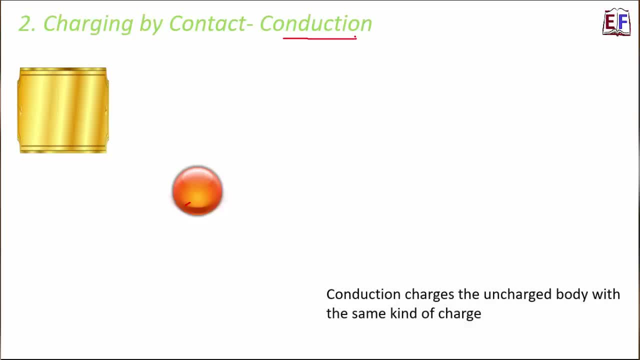 substance, it gets charged. So that's the concept. Now let us take a look at how to do this. Let us look at how this charging happens. Now let us suppose this is a negatively charged object and let us suppose this one is an uncharged. 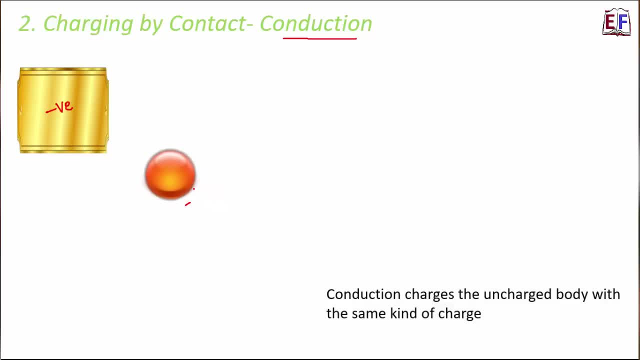 object. Now what happens when I bring this uncharged object close to this charged object? What happens? So inside this uncharged object, separation of charge takes place, Since this is negatively charged. so what happens? All the positive charges come towards this end. 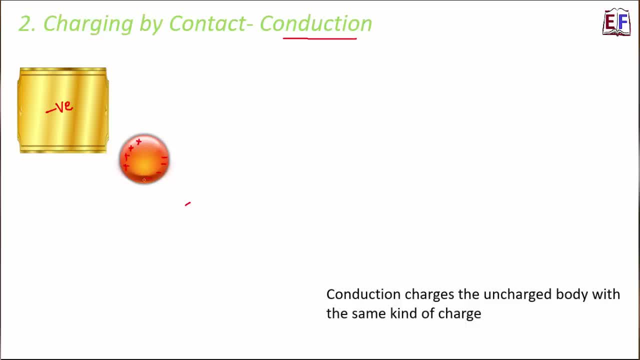 So what happens? All the positive charges come towards this end And all the negative charges go to the other end. That's because opposites attract right. So the positive charges start coming towards this end Now gradually, when this uncharged object comes in actual contact with this negatively. 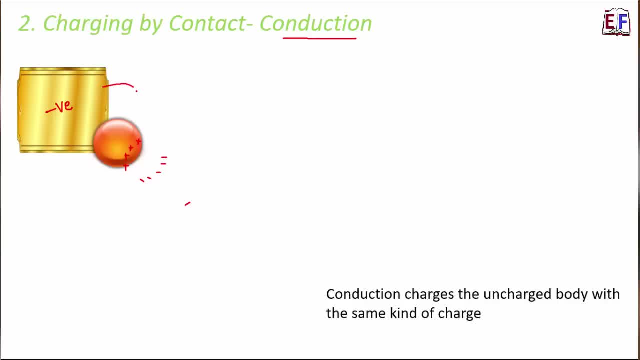 charged object. what happens? These excess negative charges move into the uncharged object. So as a result, so the negative charges move into this object. So what happens? This uncharged object becomes negatively charged. So we can say that in conduction or the process of conduction charges the uncharged body with 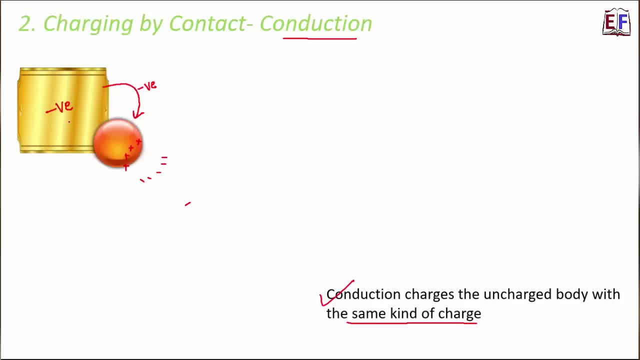 the same kind of charge. That means if this object is negatively charged, so it will charge the uncharged body negative. Similarly, let us suppose that if this charged body would have been positively charged, in that case, when an uncharged body comes in contact with it, in that case the positive 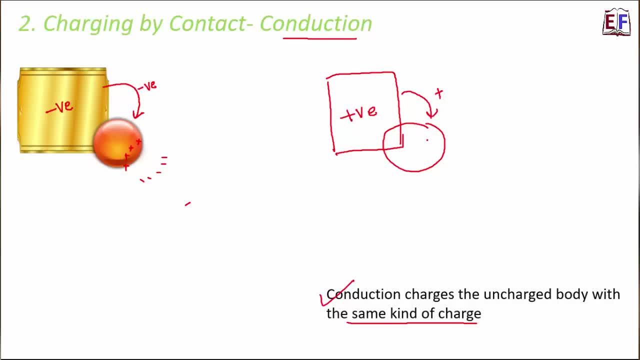 charges flow into this body and, as a result, this body becomes positively charged. right, So that's the concept. So conduction says: whenever there is charging, the uncharged body will have the same kind of charge as the charged body has. If the charged body is negatively charged, then the uncharged body will also be negatively. 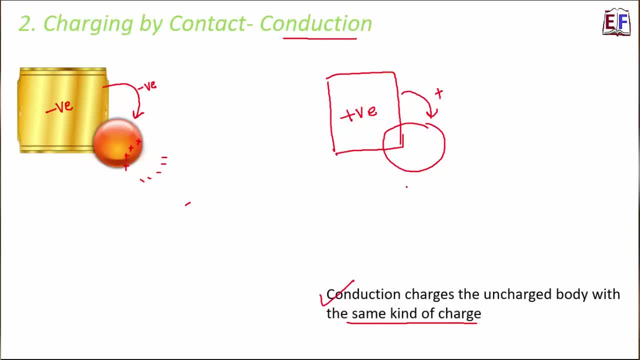 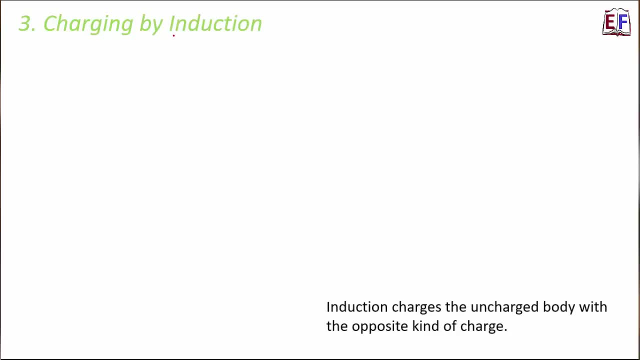 charged. If the charged body is positively charged, then the uncharged body will also be positively charged. The third method was: And the third method of charging is by induction. so in induction the object, the uncharged object, doesn't really come in contact, but it comes close to the charged object. so again, let us assume that this is a 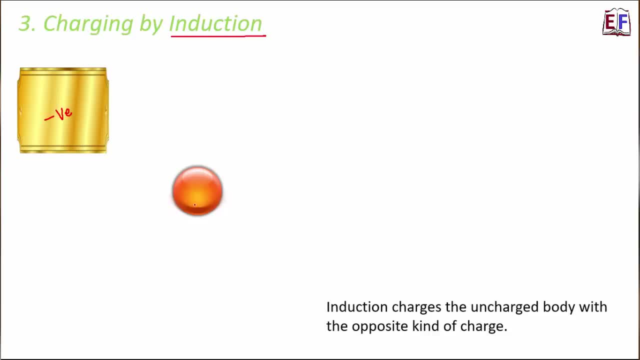 negatively charged object and this is an uncharged object. so what happens? as this uncharged object comes closer to this negatively charged object, so separation of charge takes place inside. as a result, all the positive charges they kind of settle over this surface of the uncharged body. 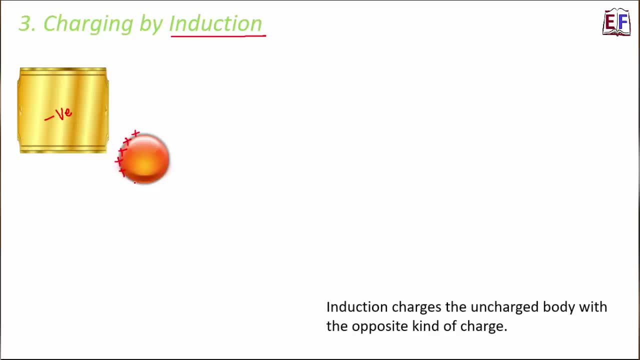 and we all know that whenever we talk about the concept of static electricity, these are those charges which kind of reside on the surface of an object, right, so that ways we can say that in this case this particular object gets positively charged. so we can say that induction charges, the 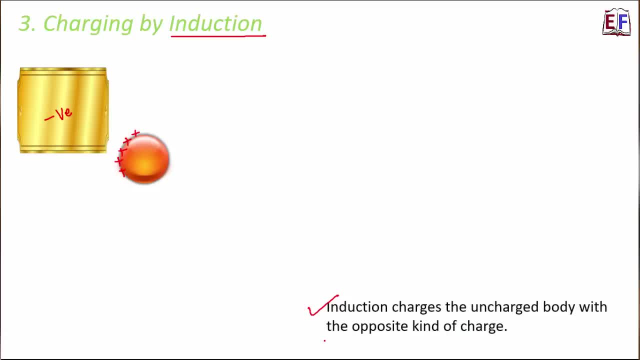 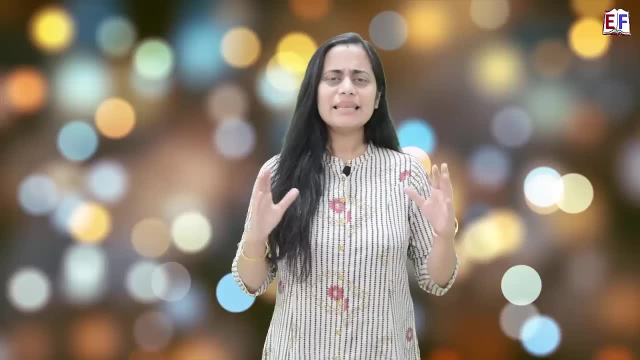 uncharged body with the opposite charge charges: the uncharged object which is non-reactive charge charges. the uncharged body which is negative charge charges the uncharged object kind of charge. so that means if this would have been positively charged, in that case this would have got negative charge. let us now look at some. 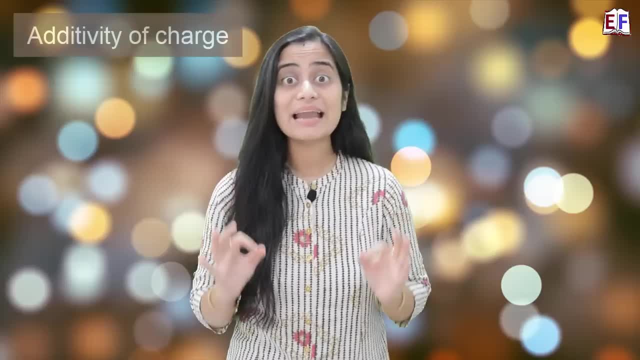 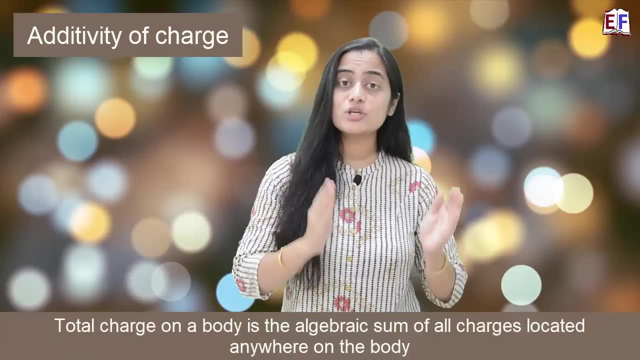 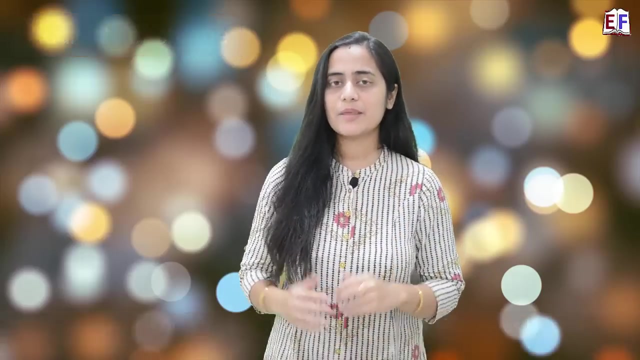 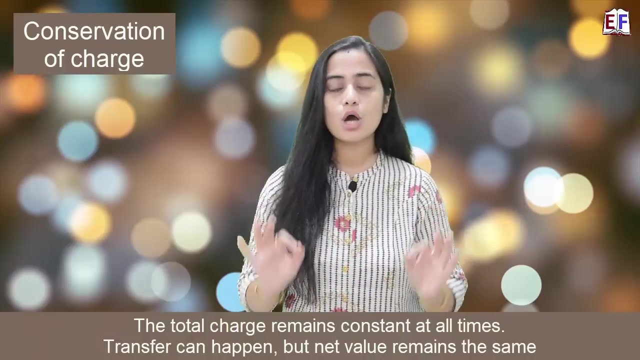 properties of electric charge. first is additive property. so what do we mean by additive property? the total charge on a body is the algebraic sum of all the charges located anywhere within the body. second, conservation of charge. in an isolated system, the total charge of the system always remains the same. now 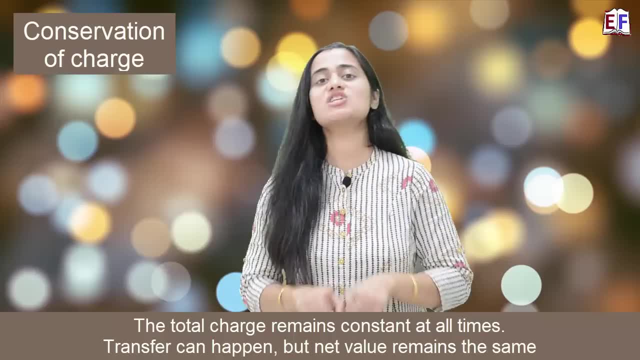 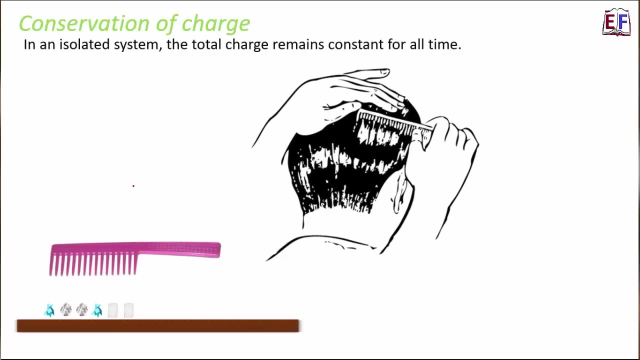 transfer of charge may happen, but the net charge within the system is always constant. for example, if we talk about the process of charging of the comb by rubbing it with the head. so in this case the total charge before must be equal to the total charge after. that means the total charge of the comb and the hair. 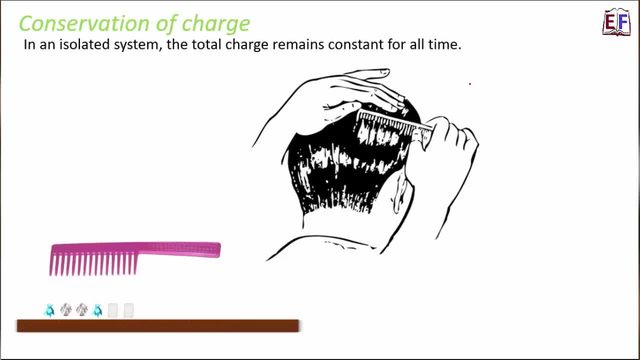 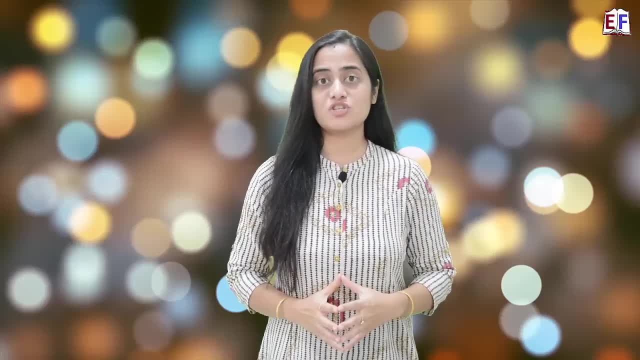 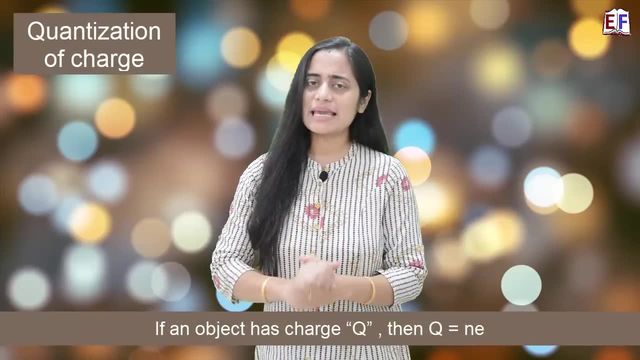 before rubbing should be equal to the total charge of the comb and the hair after rubbing. so that is what is conservation of charge, quantization of charge, a very important property of charge. what do we mean by this exactly now, whenever we say that this object has some charge, what do we? 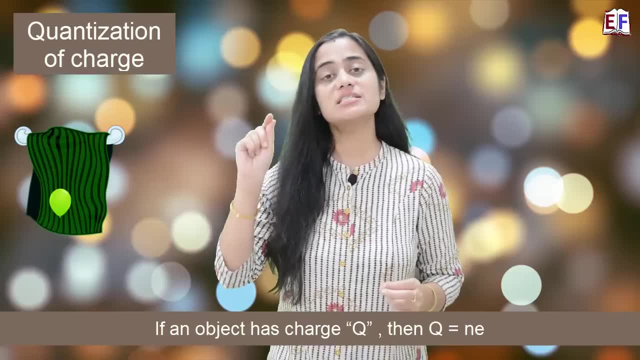 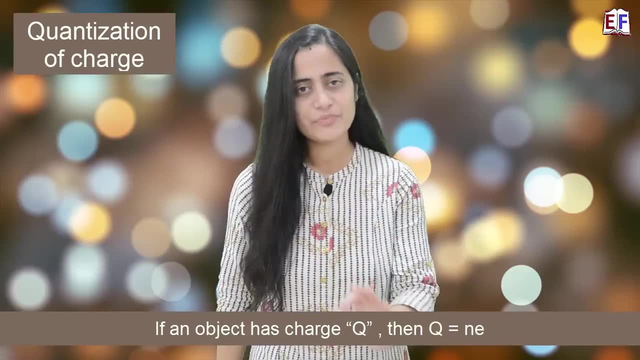 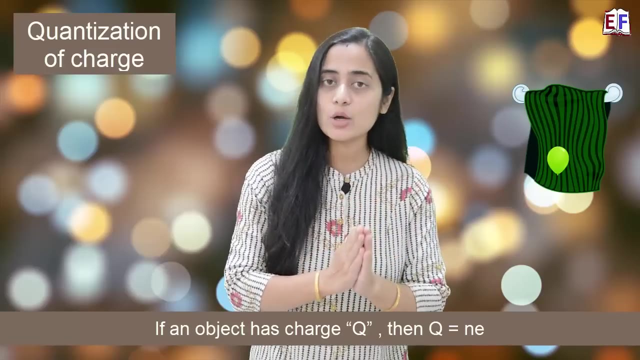 mean? we mean that that charge is basically the charge of all the electrons which are present in that object. for example, if i say that this object has charge q, so that actually means that q is equal to ne, where e is the charge on one electron and n is the total number of electrons. 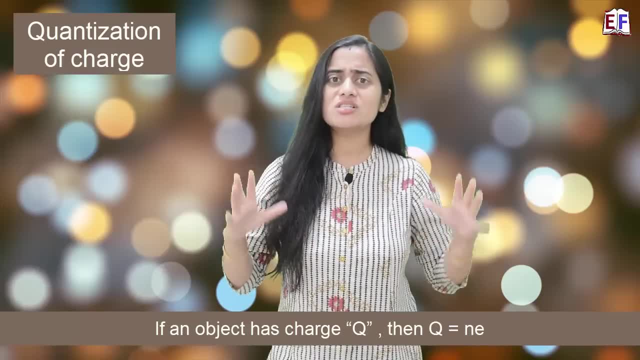 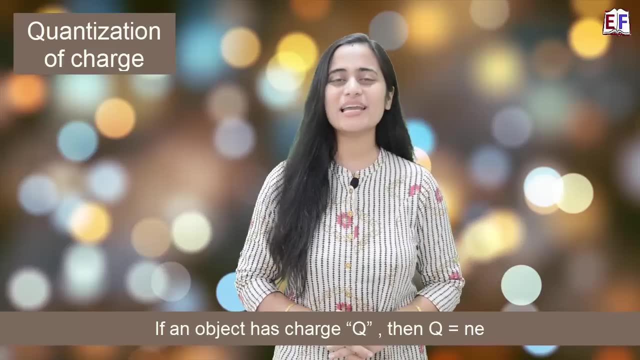 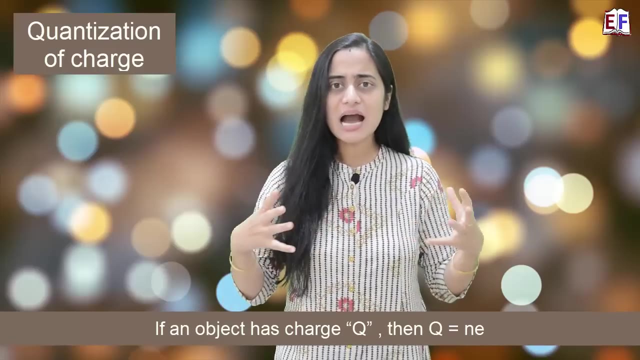 in that object. in fact, all possible charges in this universe exist in this form, that is, q is equal to ne and this is called quantization of charge. in fact, quantization of charge talks about the discrete nature of charge. charge we often, which we often see as a continuous 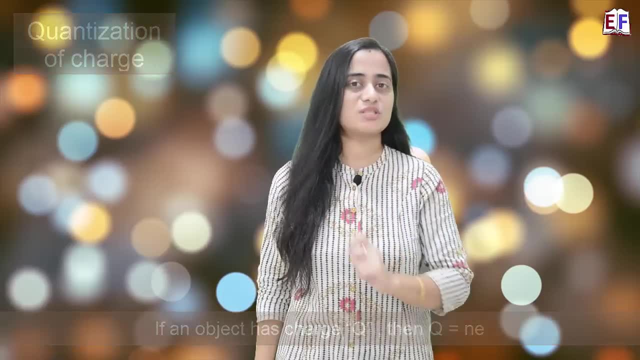 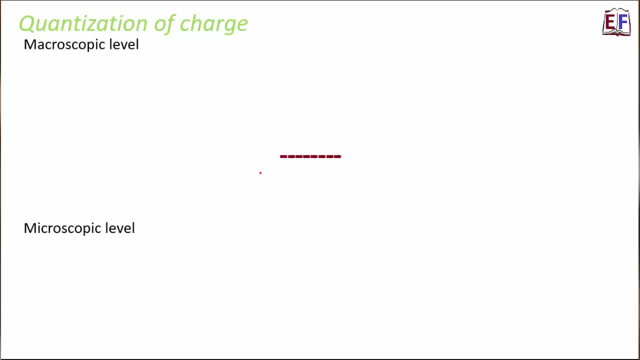 property actually exists in discrete forms. let us look at this scenario. if i ask you, what is this red thing that you see? what would you say? you would say that it seems to be a straight line, right. but now, when we go deep into it to analyze what exactly it is, you know, what do we see? we see. 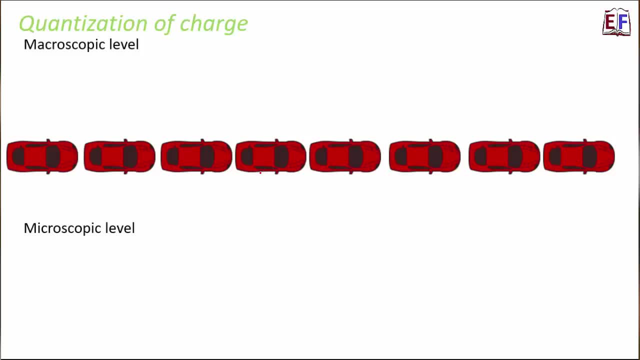 that it is actually many red cars which are, you know, standing one beside another. so what happened? our perspective changed. so when we were looking at the same thing from a very far away distance, i would say at a macroscopic level, it looked like a straight line. but when we went deep down and went, 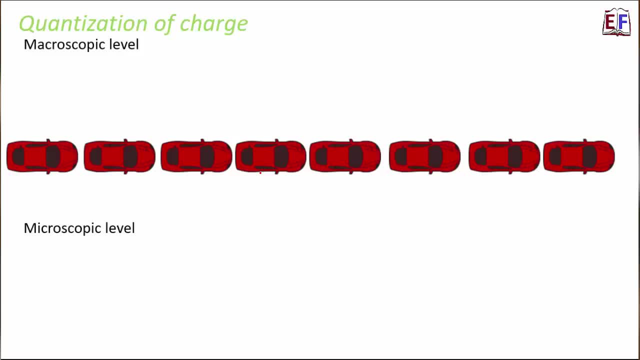 inside it to see what it is at a microscopic level. we found that it was not a straight line, rather it was a collection of many different cars. in a similar way, when we talk about charge and when we look at it at a macroscopic level, it seems to be continuous because we often say: right the charge on this. 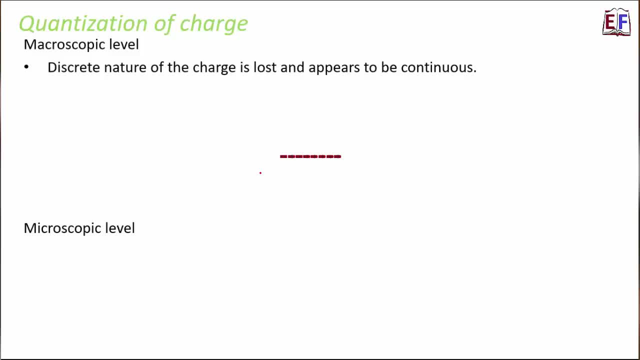 object is the five coulombs, the charge on the surface of this object. so it seems as if, okay, charge is all over and it is a continuous thing, right. but actually when we look at it at the microscopic level, we see that it is discrete in nature. so if we say that a particular object has 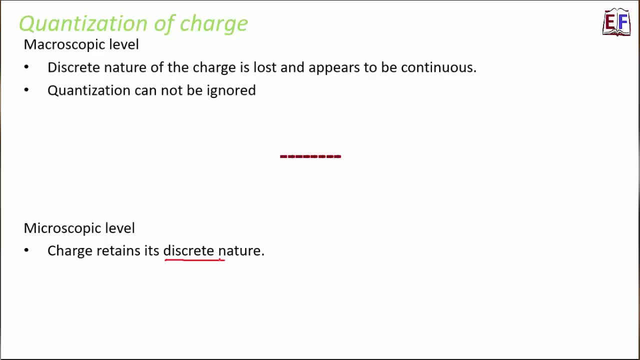 this much charge? that actually means that it has the total charge of all the number of electrons that it has. is this much right? so basically, it is discrete in nature, but in any of these cases quantization cannot be ignored. so at a macroscopic level also, it seems as if the discrete nature is. 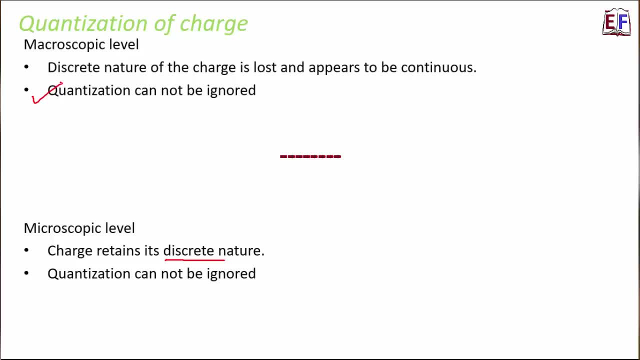 lost, but actually it is discrete in nature. so it is discrete in nature, so it is discrete in nature. actually the discrete nature is not lost and obviously at microscopic level the quantization cannot be ignored. so quantization of charge is universal coulomb's law, a very important law, very 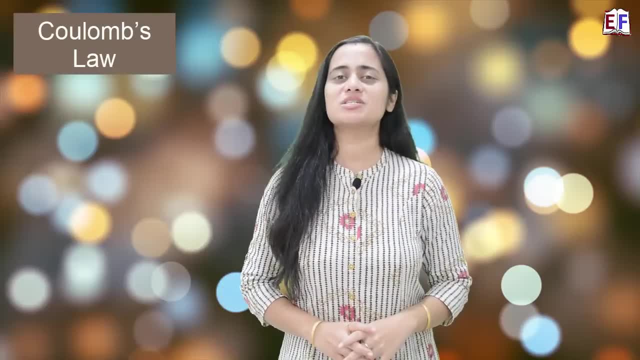 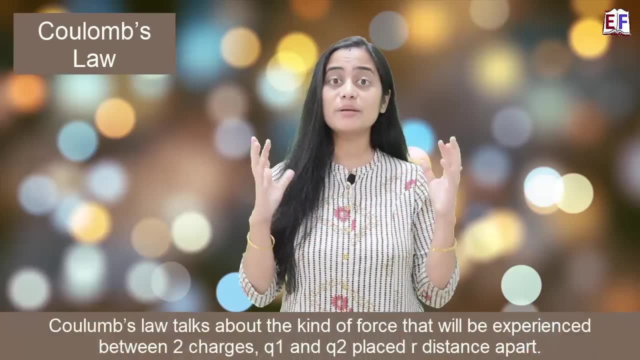 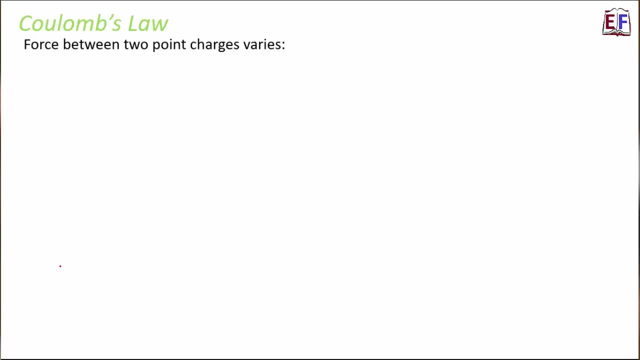 important from your exam perspective as well. you often get questions or numericals based on coulomb's law. so coulomb's law talks about the force experienced between two charges, say q1 and q2, which are placed our distance apart. coulomb's law states that the force between two point charges- let's denote that as f- varies. 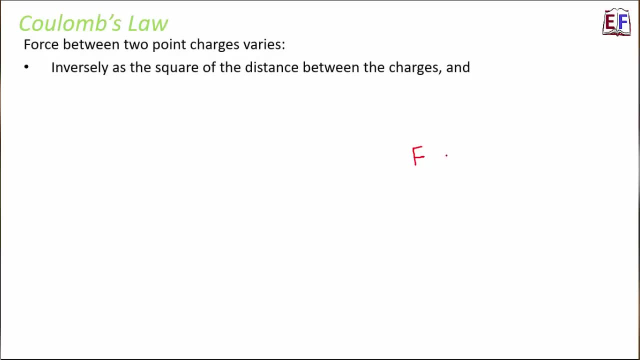 inversely as the square of the distance between the charges. so let us suppose that there are these two charges, let's say q1 and q2, and they are distance are apart. so this law states that it is inversely proportional to the square of the distance between the charges. it is directly. 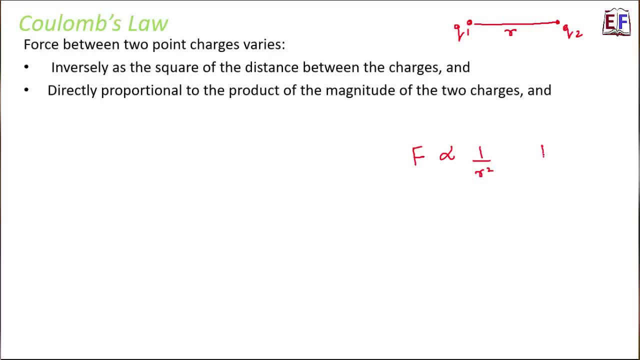 proportional to the product of the charge and it is inversely proportional to the product of the magnitude of the two charges. that means it is directly proportional to q1, q2 and it acts along the line joining the two charges. so that means the line, this line which is joining these two charges. 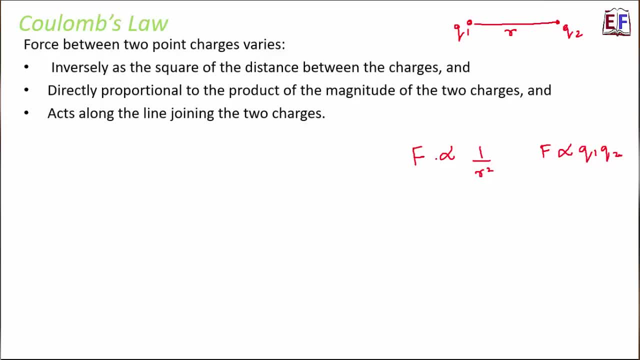 this force will also act along this line. so, based on these three criteria, it is found that force is proportional to q1, q2 by r square. to convert it into equality, we introduce a constant and we call this constant as k. so k is some arbitrary constant. so how do we later calculate the value of k? so 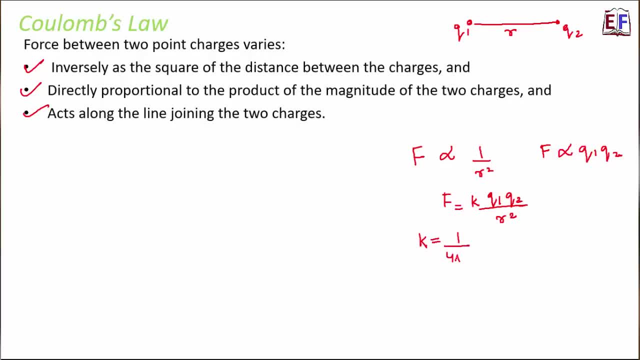 later k was calculated as 1 by 4 pi, epsilon naught, where epsilon naught is permittivity of free space. so epsilon naught has a constant value of 8.85 into 10 to the power minus 2. so epsilon is equal to 12 coulomb square per newton per meter square. so putting that value, k was found. 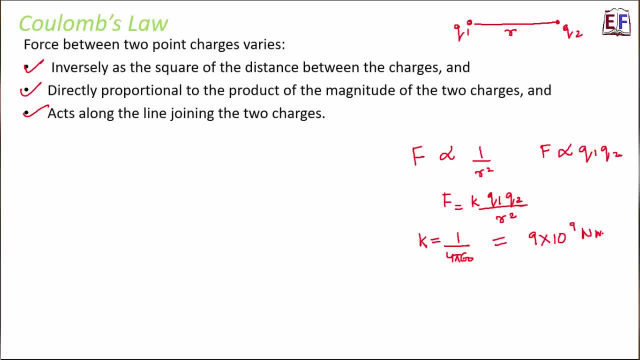 to be 9 into 10 to the power, 9 newton meter square per coulomb square. so in this fashion we derived coulomb's law, so we arrived at coulomb's law. so this expression tells us what will be the force experienced between the two point charges which are placed are distance apart. 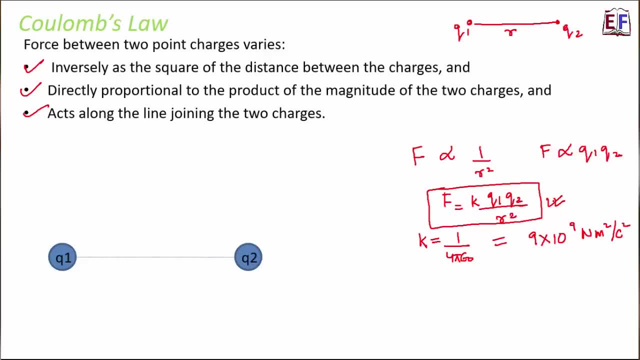 now let us suppose that if these are the two charges, q1 and q2 are equal to the force experienced one and q2. and let us say that both of these charges are opposite in nature- for example, one is a positive charge, the other one is a negative charge- then what happens? attraction. so they come. 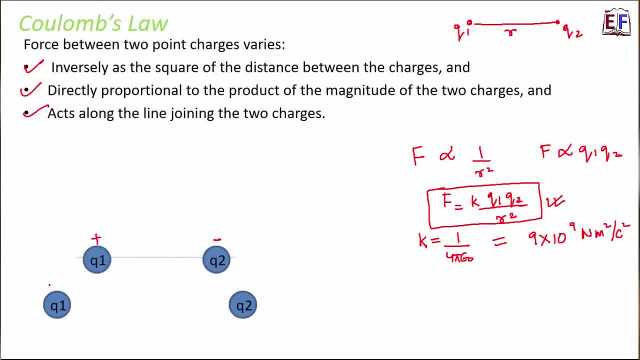 towards each other, whereas if both of these are like charges, as in, this is also positive, and this is also positive, then what happens? they tend to go away from each other because, like charges repel, but in any case this force acts along the line that joins these charges. so when we talk about 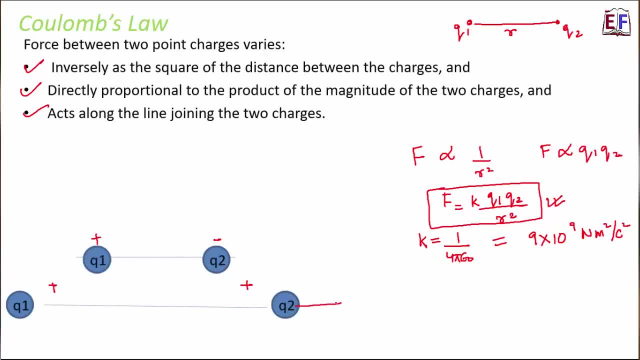 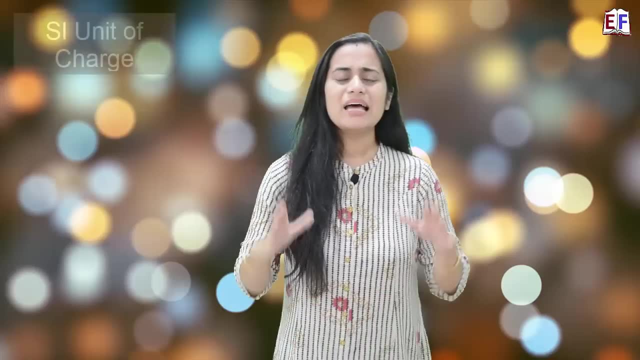 like charges, since they move away from each other, therefore, the force acting on each of these charges would be in the outward direction. but when we talk about unlike charges, since they attract, therefore, the force experienced would be in the inward direction for both of them. right now that we got an idea about coulomb's law, 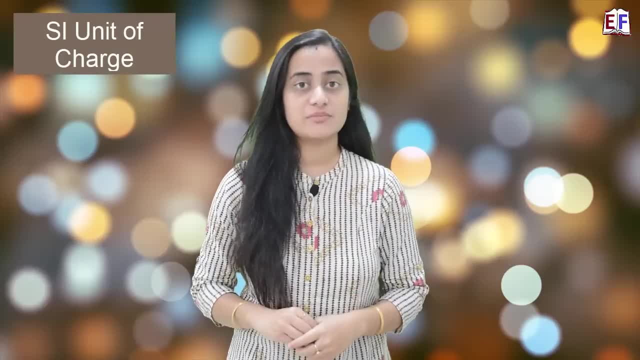 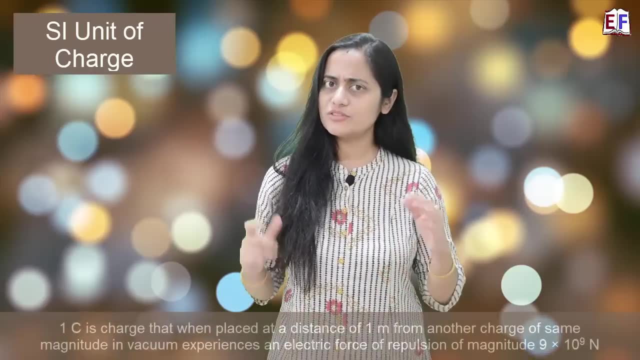 it's time to talk about the force acting on the line that joins these charges. so let's talk about coulomb's law. it's time to introduce the si unit of charge. and what's that? it's coulomb denoted by a capital c. and how do we define one coulomb? obviously using coulomb's law. so one coulomb of 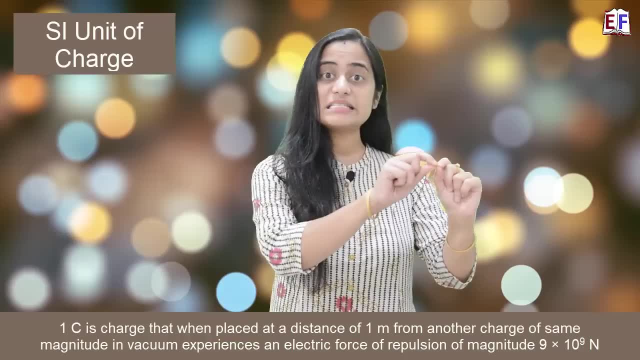 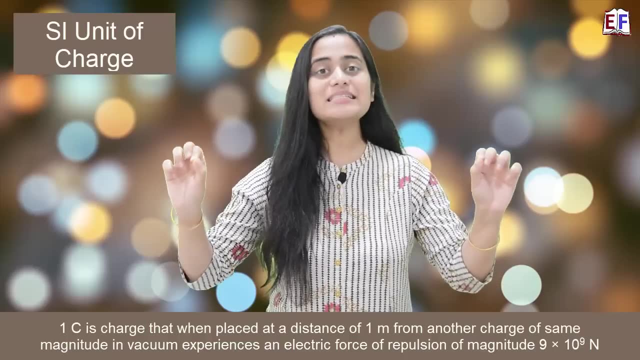 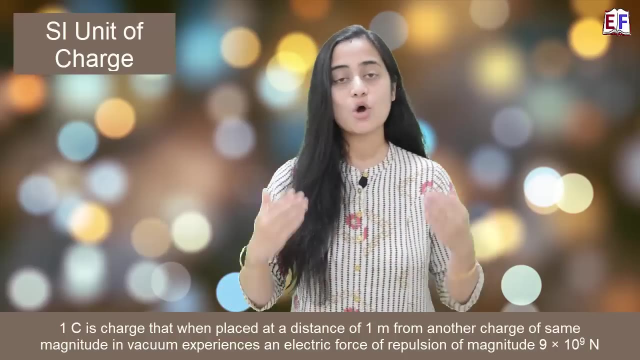 charge is that charge which, when placed at a distance of one meter from another charge of same magnitude and same type, experiences a force of 9 into 10 to the power 9 newton. very simple, you can directly apply coulomb's law and see this: one coulomb charge, one coulomb charge. distance between them is one. 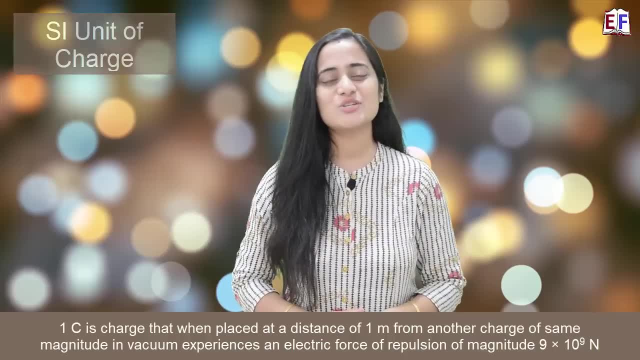 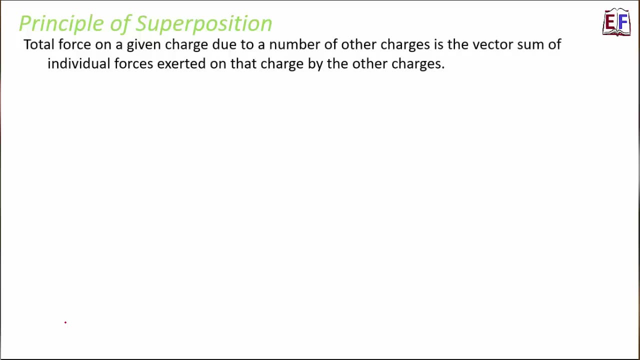 meter. so what will be the force experienced? 9 into 10 to the power 9. newtons principle of superposition states that total force on a given charge due to a number of other charges is the vector sum of the individual forces exerted on that charge by the other charges. now let us look. 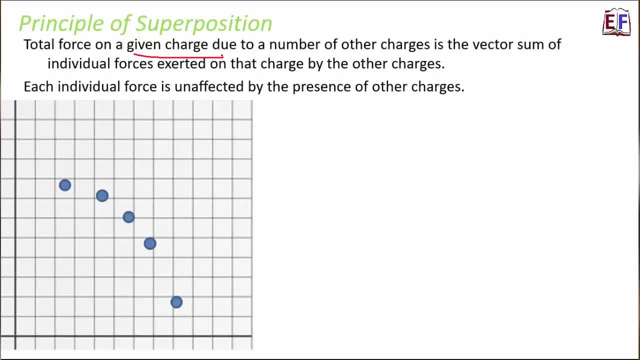 at it in this way. let us suppose these are some of the charges that are exerted on that charge. let's say q1, q2, q3, q4, q5 and so on till qn. so you have multiple charges right now. let us suppose we have to find out the total force on one charge. let us say the total force on charge q1 due to all. 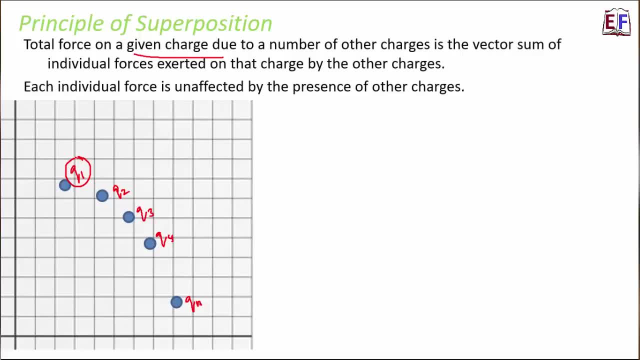 of these charges. so how will we calculate that? so this principle states that the total force on q1 would be the vector sum of the force on q1 due to each charge. so let's say q1, q2, q3, q4, q5 and so on. 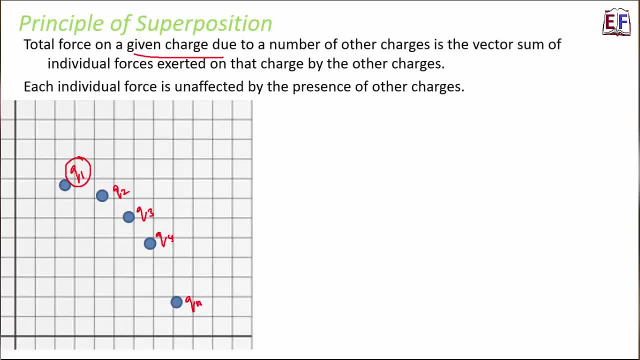 each of these charges, that means force on q1 due to q2, force on q1 due to q3, force on q1 due to q4, and so on, and sum of all of these forces, so that would be the total force on q1, correct, okay? so let's try. 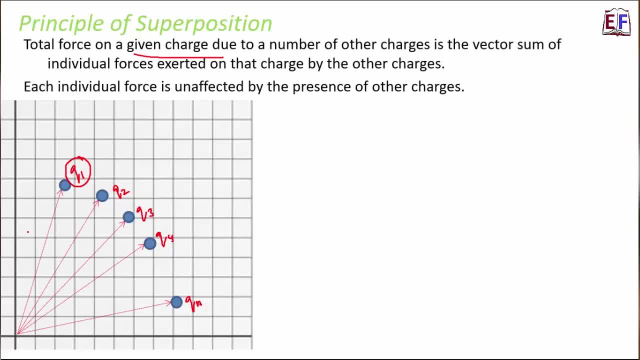 to do it a bit more. so let us suppose that the position vectors for each of these charges are given by r1, r2, r3, r4 and so on till rn. okay, so now let's try to do it a bit more. so let's suppose 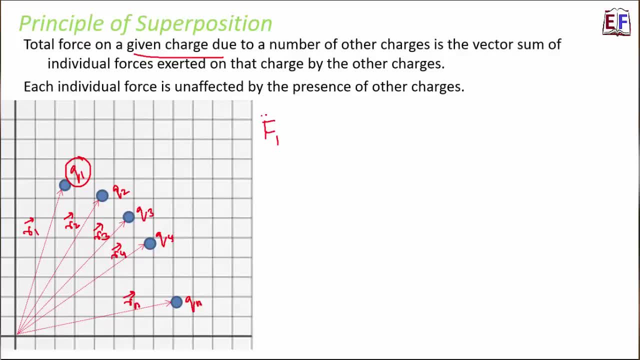 that the position vectors for each of these charges are given by rn. okay, so let's try to do it a bit more. so let's now what will happen. the net force on q1, which is denoted by f1, will be equal to force on one due. 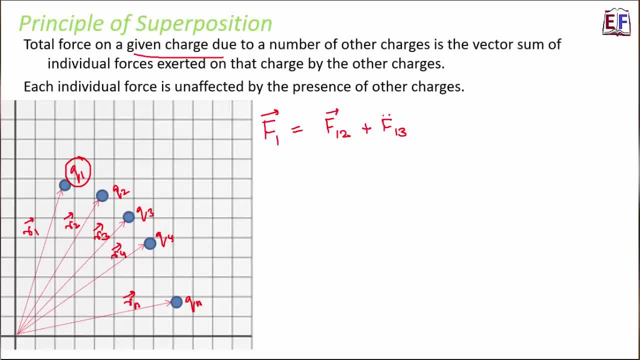 to 2, plus force on one due to 3, plus force on one due to 4, and so on till force on one due to n, and how do we calculate each of these values? so it also says that each individual force is unaffected by the presence of other charges. now, when we are calculating the force on one due to n, we are: 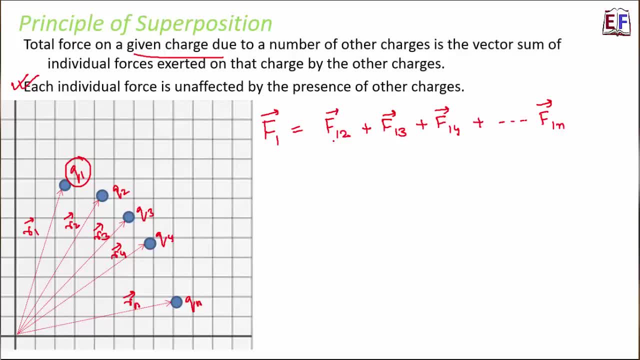 calculating the force on one due to two. we can simply apply coulomb's law, because it doesn't get affected by the fact that there are so many other charges as well in the background. that doesn't matter. so how do we calculate each of these values? for example, force on one due to two will be equal. 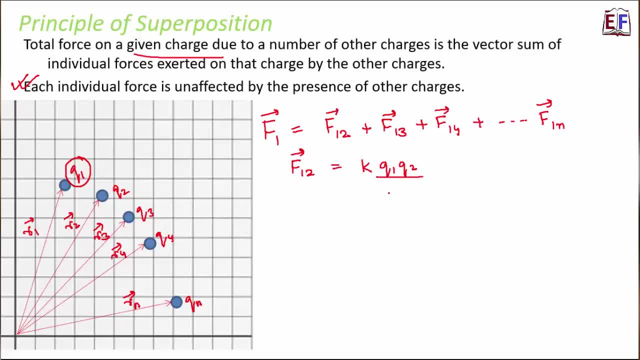 to kq1, q2 divided by r21 square, where r21 is the distance between these two charges. and here we are dealing with vector. therefore this unit vector right. so in a similar way, we will have values for each of these forces and their vector sum will give the total force on charge. 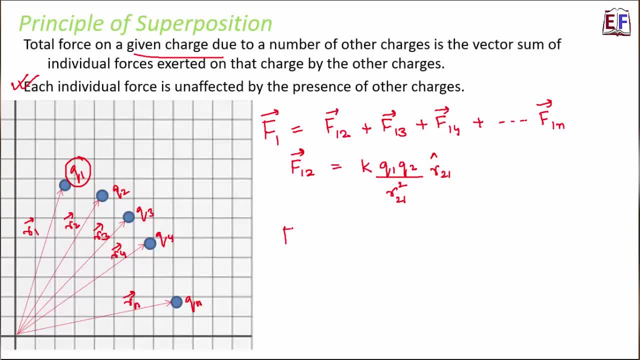 q1. so in general we can say that force on any charge qi is given by k, summation of qi, qn divided by r square, ni, r ni, unit vector. now it looks complicated, but actually i have written the same thing just in terms of a generic. you can say a general formula, right? so if you put the 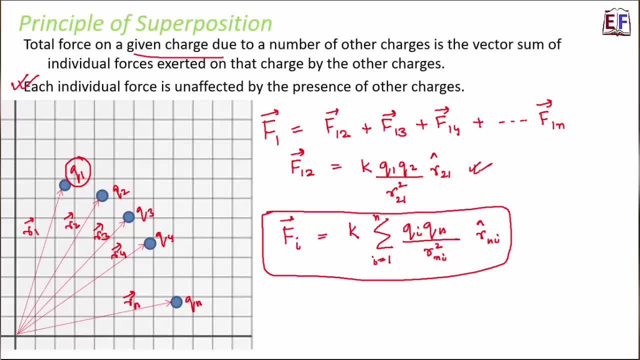 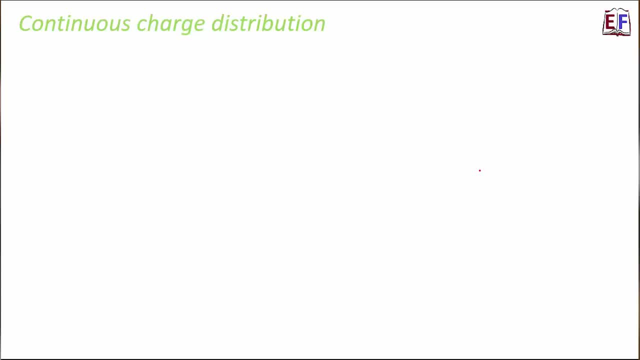 value of i as one. this is what you will get. continuous charge distribution. charge is still discrete in nature, just that the distribution is continuous. so extremely closed space charges form continuous charge distribution. so when we talk about continuous charge distribution we talk about three things. one is linear. second. 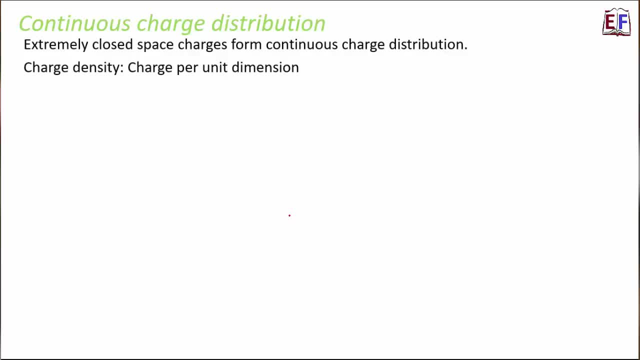 two is linear, third is linear, fourth is linear, fifth is linear, sixth is linear. sixth is linear, second is superficial and third is volumetric. so we basically talk about charge density rather than a discrete value of charge. we talk about the density, that is, charge per unit dimension. now 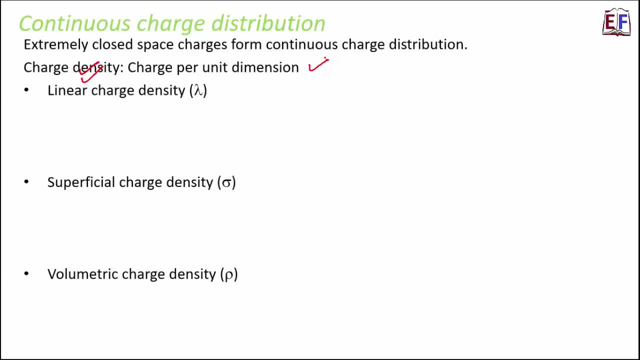 this, the dimension keeps changing. for example, if i am talking about linear charge density, which is generally denoted by lambda, this is charge per unit length. if i am talking about superficial charge density, which is denoted by sigma, this is charge per unit length. if i am talking about volumetric charge density, where i am dealing with volume denoted by rho, then 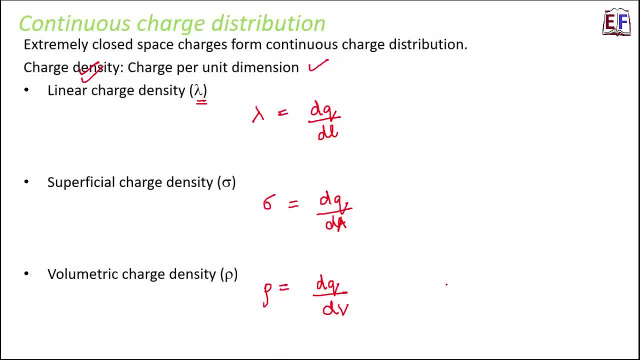 i am talking about charge per unit volume. now, when does all of these come into picture? volume comes into picture when i am looking at something which is three-dimensional, for example a cube or a cuboid, so we talk about the volume inside it. superficial when we are talking about area, a square, just just. 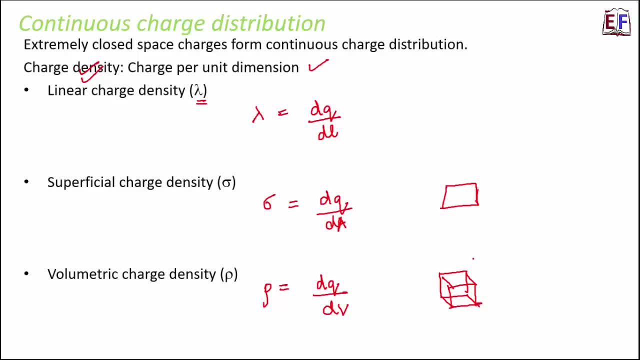 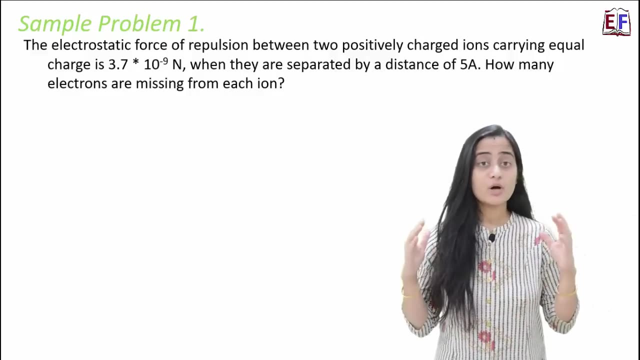 one surface of this cuboid could be an area, linear when we are talking about a line, for example, a thin rod. so that's where we talk about linear charge density. lot of theory, we have read a lot of theory, and let's look at some numericals, because just now i said that coulomb's law is very important from exam perspective. 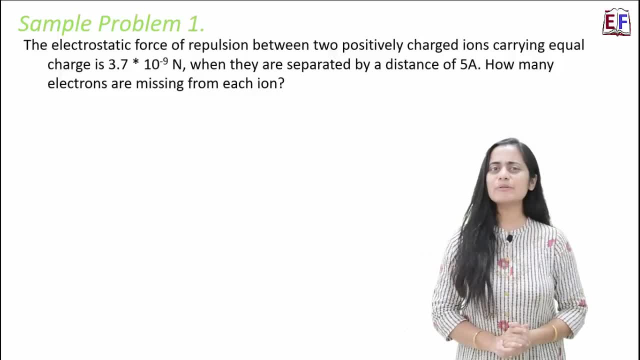 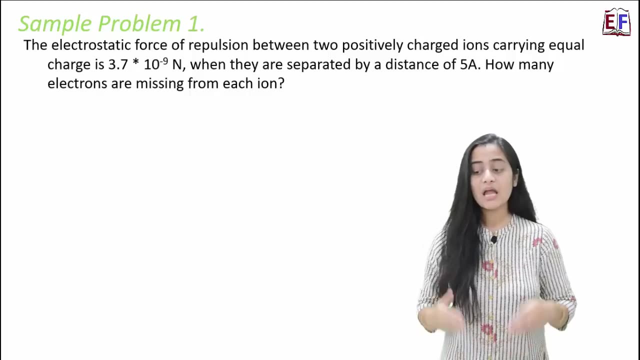 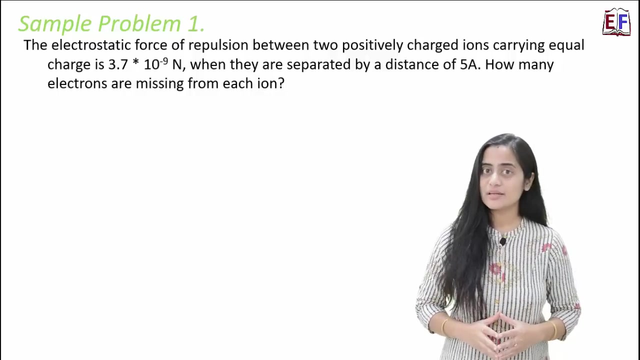 that means from this numericals can come. so let's look at a sample problem. sample problem number one: the electrostatic force of repulsion between two positively charged ions carrying equal charges is three point seven into ten to the power minus nine newton when they are separated by a distance of five angstrom. how many electrons are missing from each ion in this? 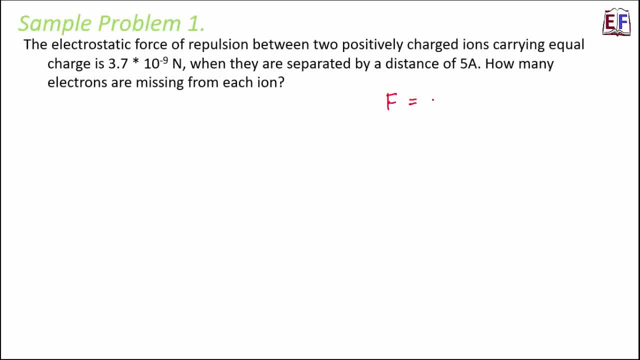 case, the force between these two charges is given as three point seven into ten to the power minus nine newton, and the distance between the two charges is five angstrom, which is equal to 5 into 10 to the power minus 10 meters. now we have to find out how many electrons are missing from each ion, so the for our in order to solve. 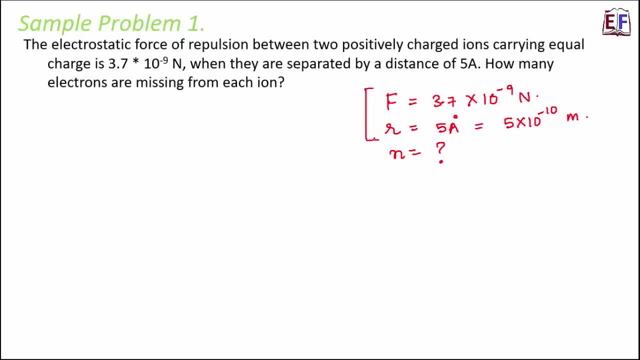 this question. our first step would be to find out the dimension of the charge. i mean, we have to find out the value of the charges, because here the situation is such that this is a positive charge. this is another positive charge which is separated by distance r now, since both of these are positive, 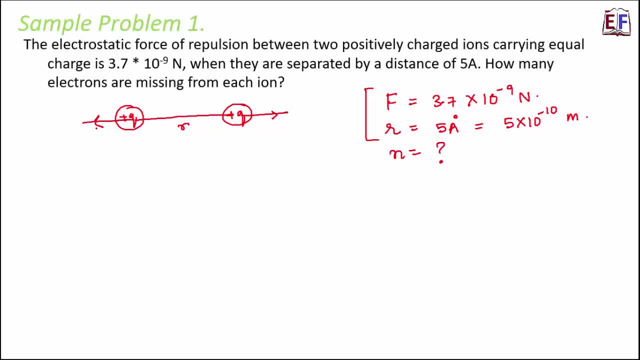 they will repel in this fashion correct. now, from coulomb's law we know that f is equal to k, q1, q2, which is q square divided by r square. so therefore q square will be equal to f, r square divided by k. f is given, r is given, k is a constant which is 9, into 10 to the power 9. so we will put all of 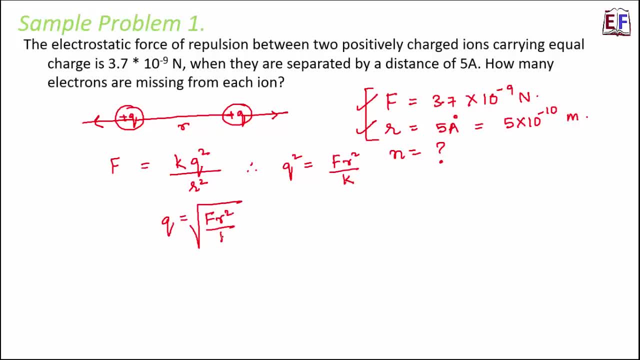 these values here, so this becomes equal to root over. f is 3.2. 3.7 into 10 to the power minus 9. r square would be 5 into 10 to the power minus 10. whole square divided by k, that is 9 into 10 to the power 9. so this comes out to be 3.2 into 10 to the power. 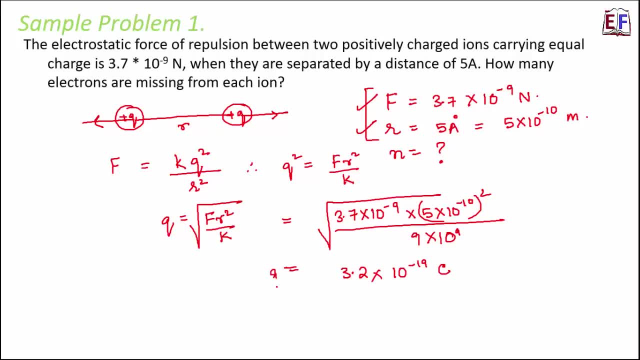 minus 19 coulomb. so that's the value of q. but we have to find out how many electrons are missing from each ion. so from the concept of quantization of charge, we know that. how can we represent charge? charge is basically the number, the total charge of the total number of electrons in that particular. 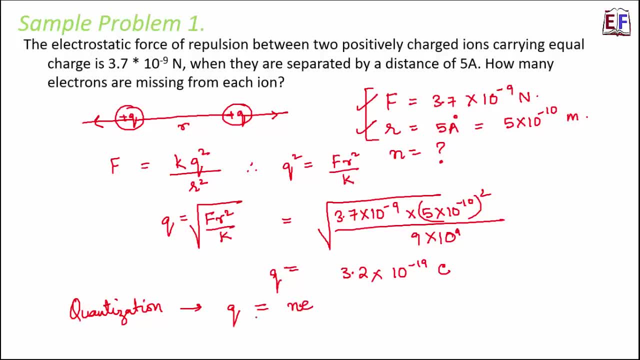 object. so this is equal to n, e. so n, that is the number of electrons, will be equal to q divided by e, which is equal to 3.2 into 10 to the power minus 19, divided by 1.6 into 10 to the power minus 19. 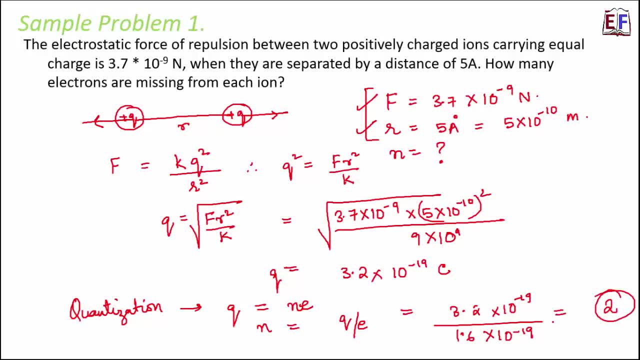 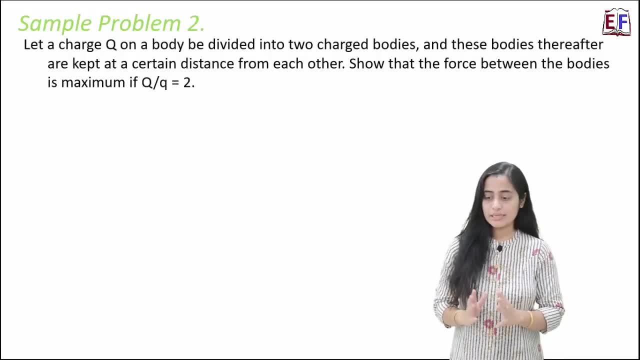 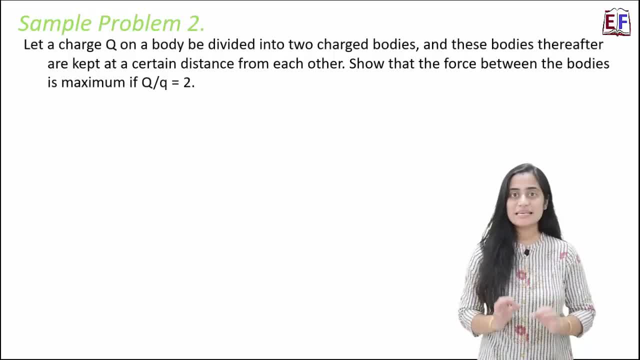 if capital q by small q is equal to 2, assume that these two charged bodies are q and capital q minus small q, because if one is small q, the other has to be capital q minus small q. right, the question says that this is q and this is capital q minus small q, and they are separated by: 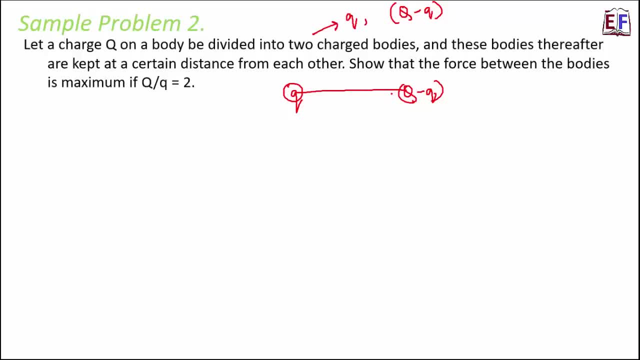 a certain distance from each other. right, we have to show that the force between them is maximum if q by q is 2.. so first of all, we need to find out the force between these two charges, which will be equal to k into q1, q2 divided by r squared right. so this is equal to q by q, is equal to q minus q minus q, and this is 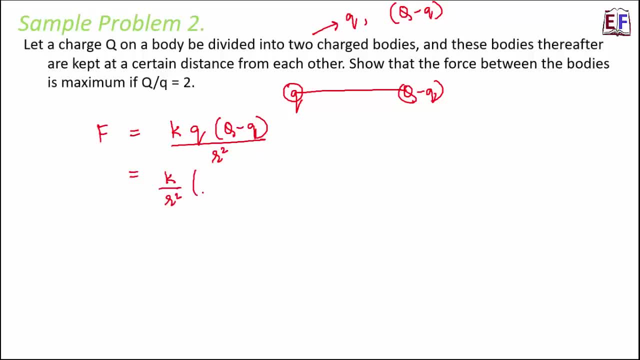 k by r square into q, q minus q square. so that is the force. now, what do we want? we want to look at the maximum value of f, that is, we want force to be maximum, therefore, and we want for maximum value of force what should be the value of q, that is, the small q. so, therefore, what we will do, we will. 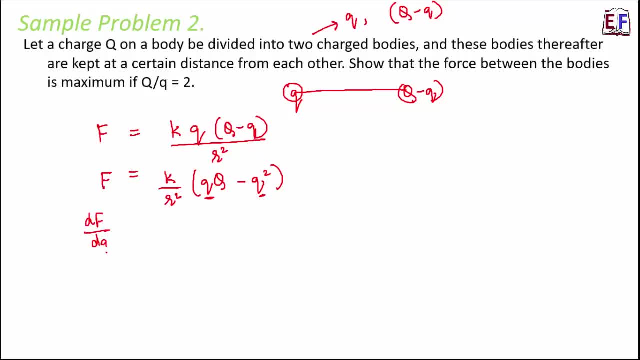 differentiate it with respect to q. so this is something which you have already learned in your differentiation integration in mathematics, right? so whenever you have to find out the maximum value of a particular thing, for example, here we have to find out the maximum value of force with respect. 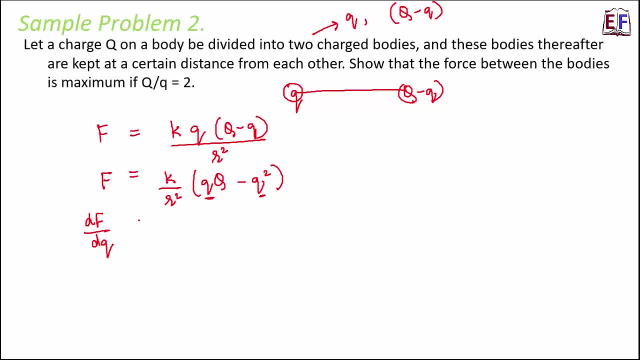 to what? with respect to this q, the value of charge, because that is what we are trying to find out, right. so df by dq. so if we differentiate it, it becomes k by r, square capital, q minus 2q. i'm not getting into differentiation concept. so now for getting its maximum value: df by 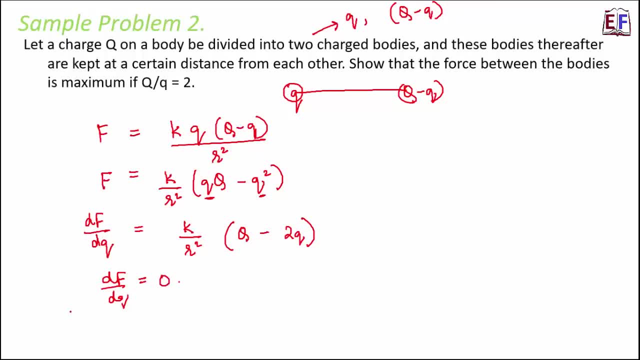 dq should be equal to 0. so therefore k by r square into q minus 2q should be equal to 0. so from this we get that small q is equal to capital q by 2. therefore, capital q by small q is equal to 2. are we done? not really, because in order to ensure, 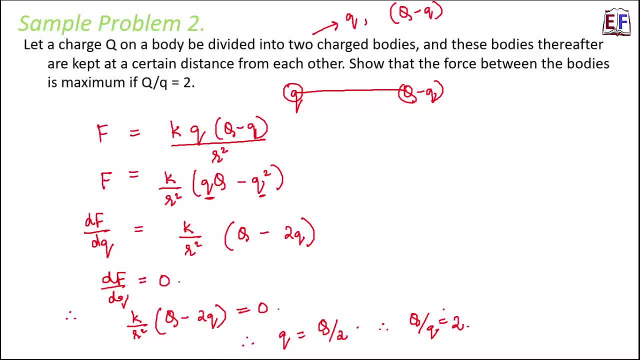 that we get the maximum value of q. we have to get the maximum value of q by dq, so we have to remember that. okay, this is the condition for its maximum value. we also need to check that at this condition, d square f by dq square should be less than 0. so that's the condition for maxima right. 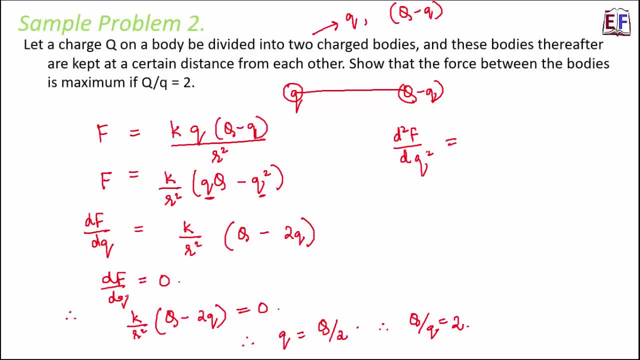 for maxima. first we say that df by dq should be equal to 0. also d square f by dq square should be less than 0. so let's calculate d square f by dq square. that will be equal to k by r square into 0 minus 2. 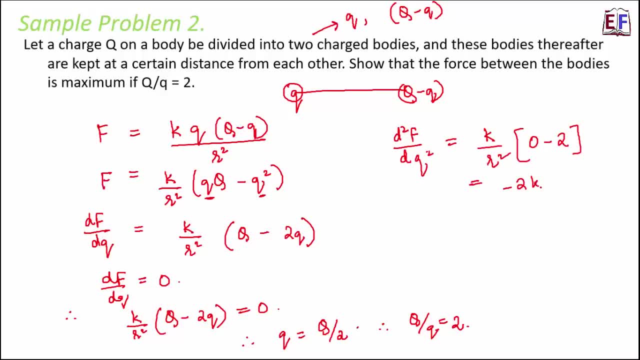 so that is equal to minus 2k by r square, which is less than 0. so therefore this is the correct condition. so here quite a bit of mathematics was involved. for all those who didn't understand it, please refer to the differentiation video. in fact, i have created a separate video for 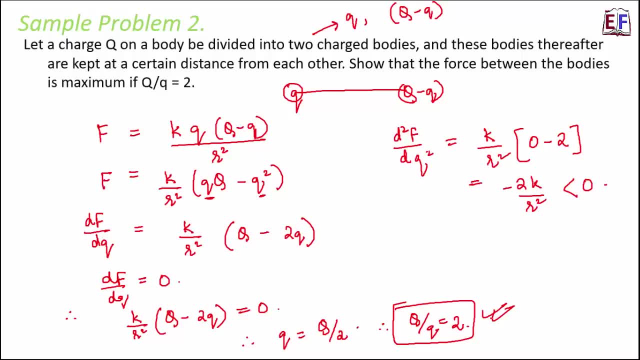 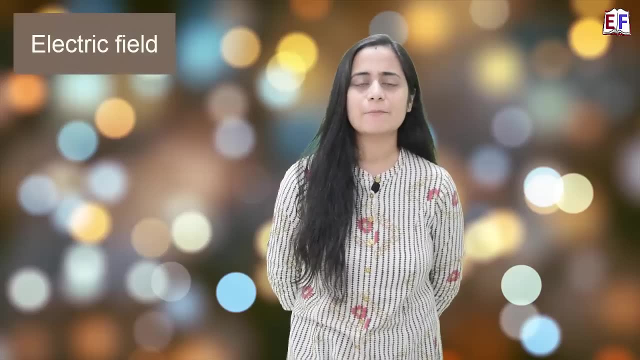 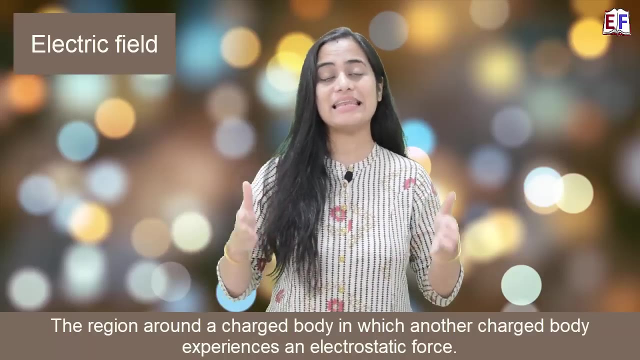 understanding, differentiation and integration for those students who do not have maths as one of their subject. and all these important links are given in the description. time to introduce the next character of the movie, and that is electric field. so what's electric field? it's the region around a charged body where another charged body experiences an electrostatic force. 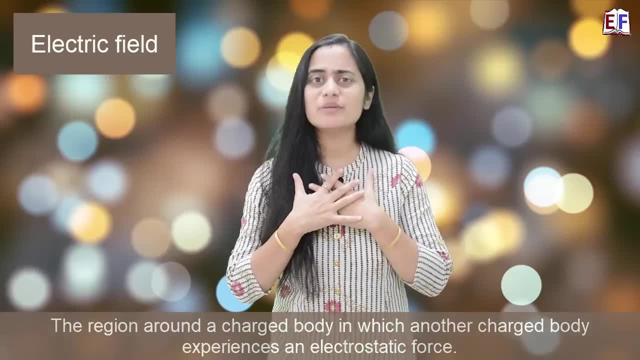 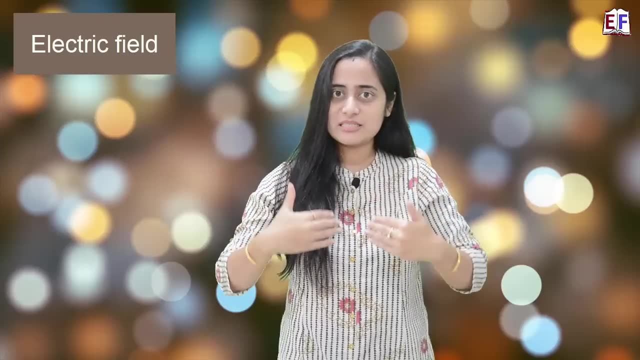 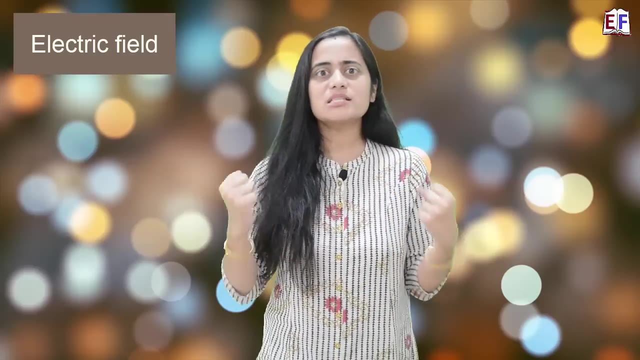 so it's like: uh, let's say that i am a charged body, so the area around me which is like my, my area. so if this is me, i am a charged body and this is my area, in which anyone will come from outside, so he will experience a different force. so that is my electric field. let's say, plus q is a charge. 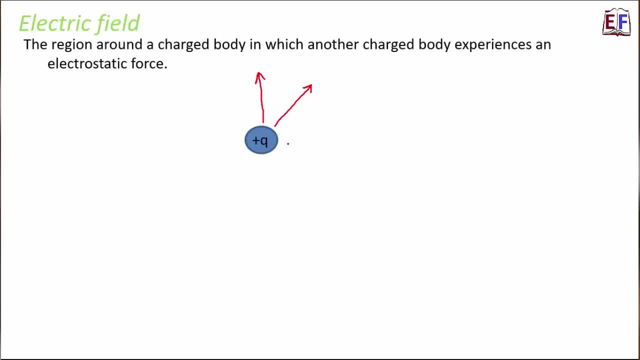 and the region around this plus q where another charge would experience a force. for example, if there is another charge, let's say q naught, so the moment q naught enters this region where it experiences an electrostatic force. so this entire region is the electric field of plus q. 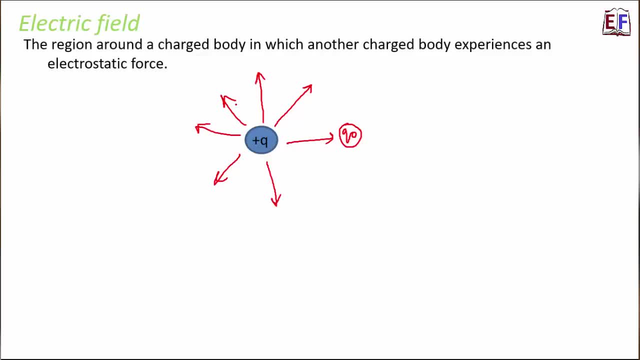 and this region is. we can say it is the range of electric field for this particular charge. now, as we talk about these concepts of electrostatics, we will very often use two words: source charge and test charge. so let me clarify right at the beginning what are they and how are. 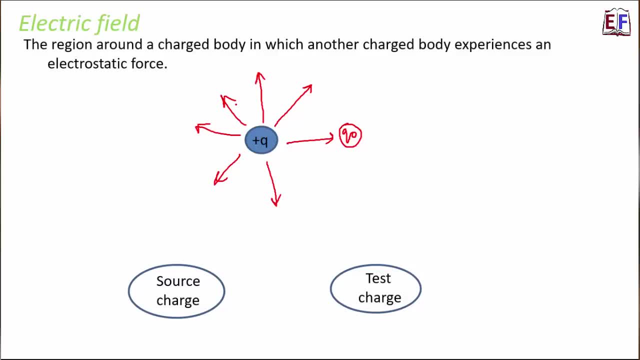 they different. so when i talk about a test charge, it is a negligibly small charge. so you can imagine it is a very, very small charge. it is a very, very small charge. so it is a very, very small charge. it is so small that it doesn't have an electric field of its own, so this charge cannot produce. 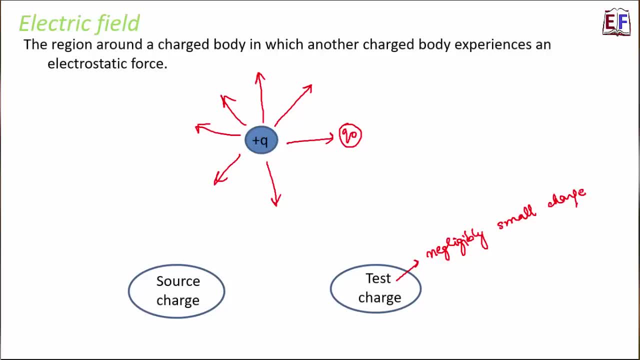 its own electric field, so it is such a small charge. but when i talk about a source charge, this charge is capable of having its own electric field. in fact, that is why it is called source charge. how will you remember which is source charge, which is test charge, source? so it is the. 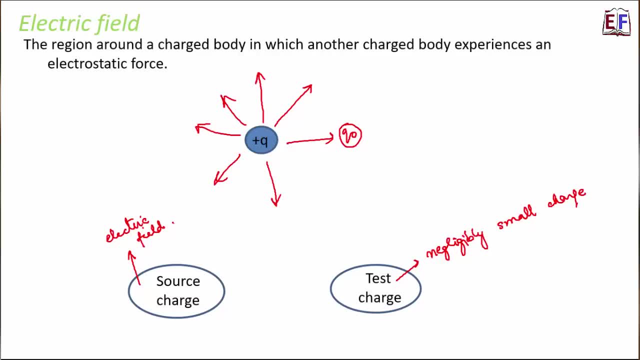 source of electric field. so this charge makes its own electric field. so in this picture plus q is a source charge because it has its own electric field. and what is q naught? q naught is a test charge, at least here, because it doesn't have its own electric. 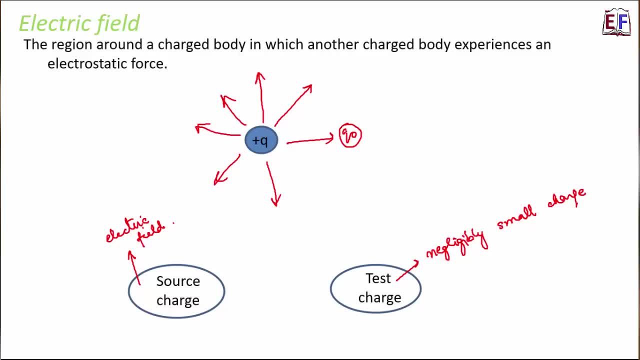 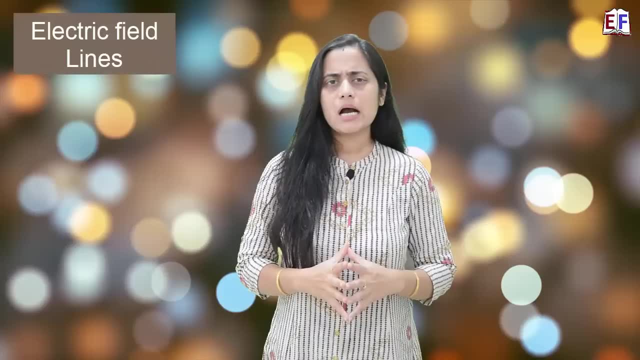 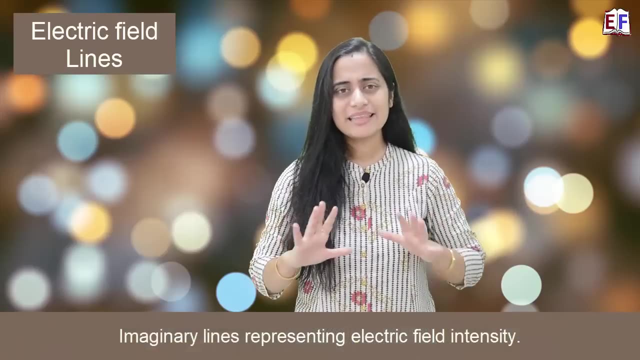 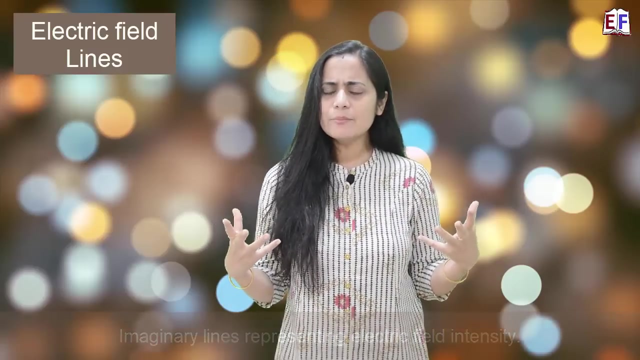 field. it is just coming and experiencing the electrostatic electric field of the source charge electric field lines. they are very important, again from exam perspective as well, but conceptually also they are very important. so what are they now? they are imaginary lines to represent the electric field. and how do we represent them? so if we talk about a positive 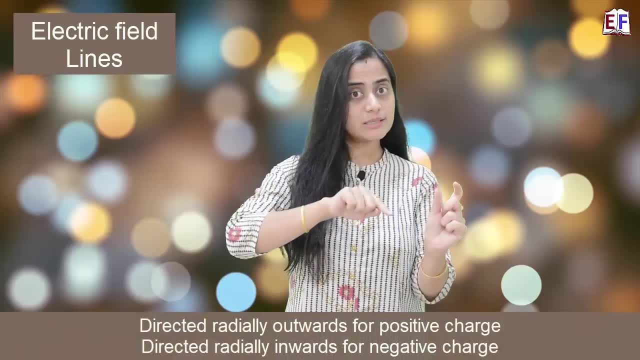 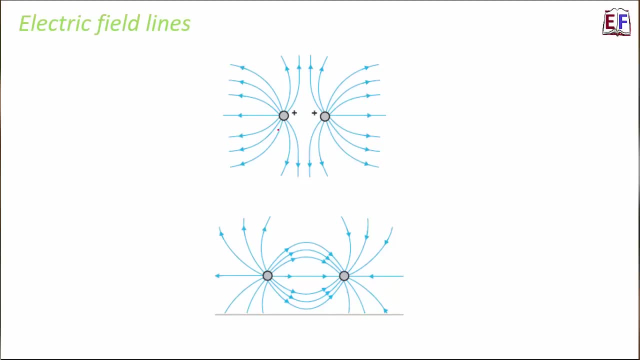 charge, they are directed radially outward. if we talk about a negative charge, they are directed radially inward. so if there are two positive charges placed like this, this is how the electric field lines would look, because the lines would originate from both of these charges, right so? 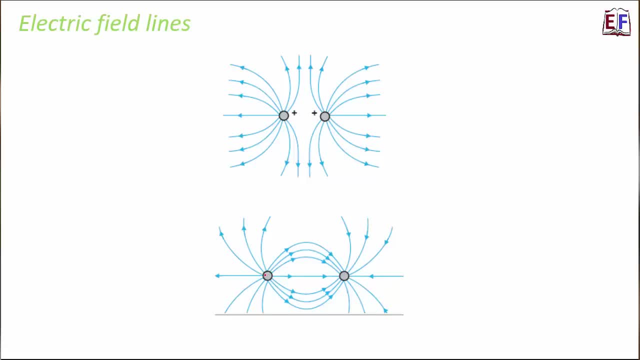 this is how they look. similarly, if you have one positive charge and two positive charges and the other one negative charge, then what happens? the lines originate from one and it terminates into the other one, as in not terminates, but it enters the other one. so that's how it. 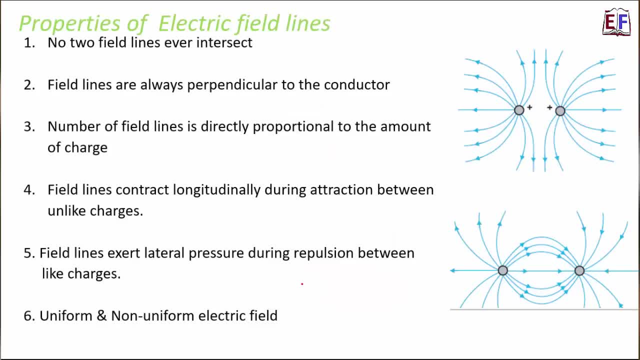 will form these kind of closed loops. let us quickly recap the properties of electric field lines. no two field lines ever intersect, because if field lines intersect, then at the point of intersection there would be two direction of the electric field, which is not possible. right, because at every point of 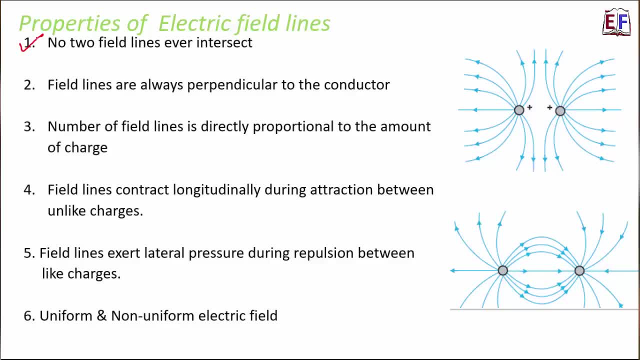 these electric field lines, you get the direction of electric field right. the second property is: field lines are always perpendicular to the conductor. third property: number of field lines is directly proportional to the amount of charge. for example, if you have field lines, just three field lines, and in another case if you have so many field lines, that means the charge, the amount. 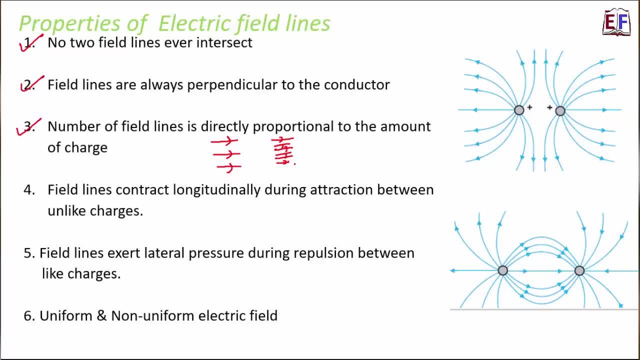 of charge in this case is very less when compared to the amount of charge in this case. fourth, field lines contract longitudinally during attraction between unlike charges. so if you look at this here, these are unlike charges, positive and negative. so in this case what happens? you can see that the field lines they contract, they are not expanding right. they 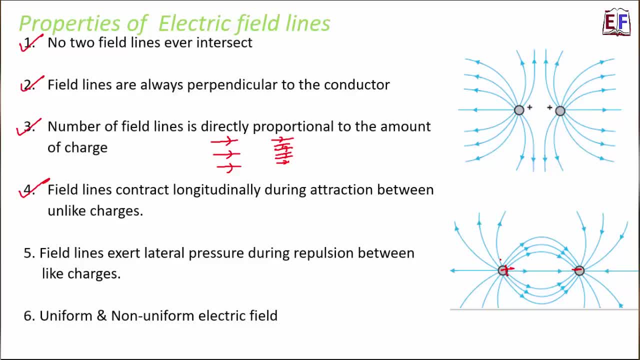 contract longitudinally because of the attraction, whereas in case of like charges, they contract longitudinally because of the attraction, whereas in case of like charges, charges, as in this case, they exert pressure on each other. as you can see, they exert some natural pressure due to the repulsion between the like charges. now here i want to add one. 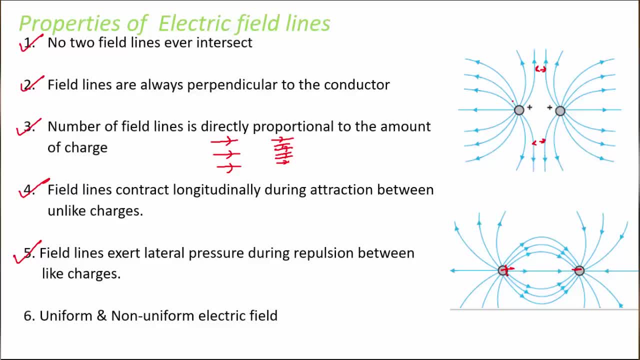 important point. so if these two charges are of equal magnitude- for example, if this is also plus q, this is also plus q- then this point, which is called the neutral point, that means this is the point where nothing is going to happen. these field lines will never touch this point. so 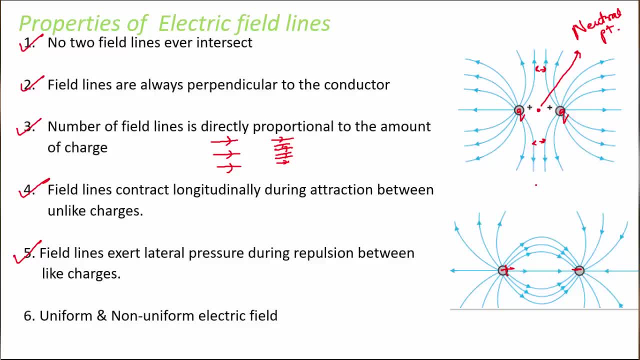 this neutral point is exactly at the center if these two charges have the same magnitude. but what if these two charges do not have the same magnitude? let us say one is plus 5q, the other one is plus q. that means one is bigger, the other one is a smaller charge. in that case, this point p, which 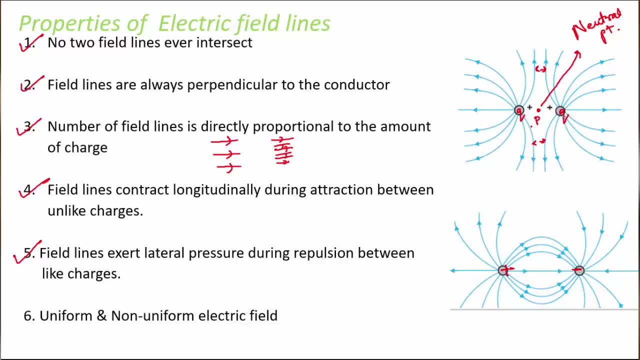 is the neutral point is not at the center and it is towards the smaller charge, because it this is how it will be. for example, let us suppose this is a bigger positive point. so if this is a bigger positive point and this is a very small positive charge, so even though repulsion will happen, but the force that 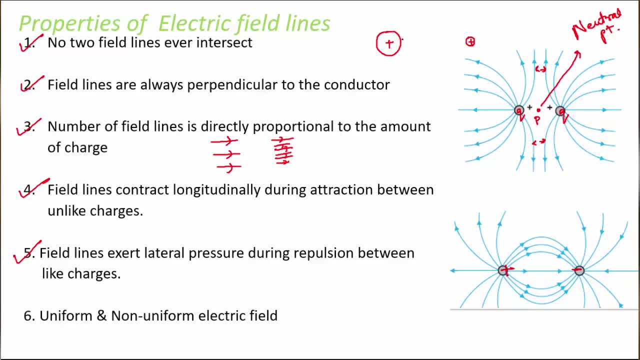 this big charge will experience because of the smaller charge is going to be very less. the small charge will have very less effect on the big charge. so, as a result, in this case, so as a result, these lines would bend very slightly correct, but this being a small charge. 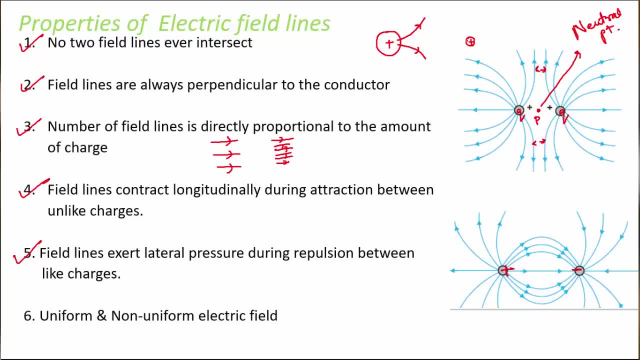 the effect that it will have because of this big charge will be huge. so, therefore, these lines would be like going totally curved right, because they will experience more force. as a result, this point p, that is, the neutral point, will shift towards the smaller charge, and that's what we try to say. 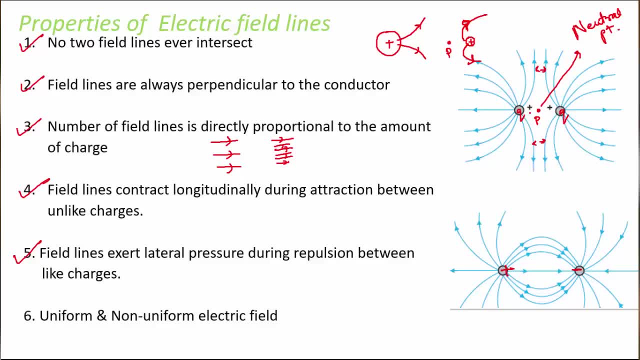 that if these two charges are not equal in magnitude, then the neutral point is always located towards the smaller charge. next is uniform and non-uniform electric field. so how do we know whether the electric field is uniform or non-uniform? just by looking at the field lines. so if we are talking about uniform electric field, then the field lines 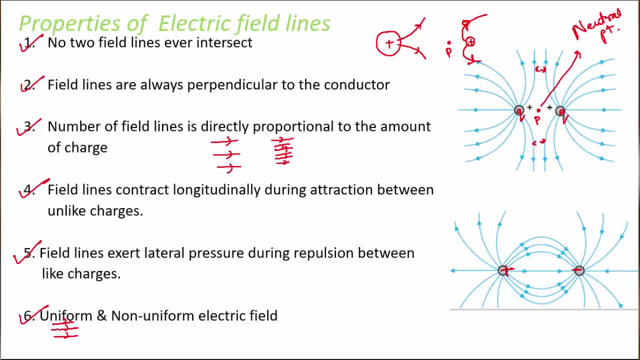 are equispaced, that is, they have equal amount of space in between. but if we are talking about non-uniform, so somewhere they will be very close, somewhere they will have huge gap, so that there you will see that non-uniformity. so these are some of the properties of electric field lines. 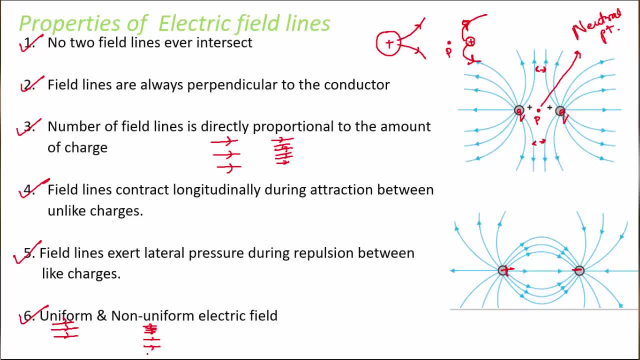 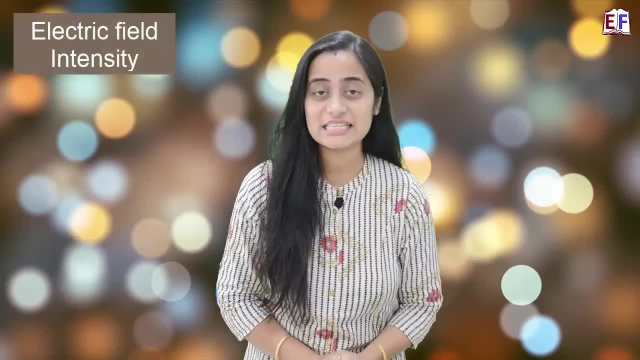 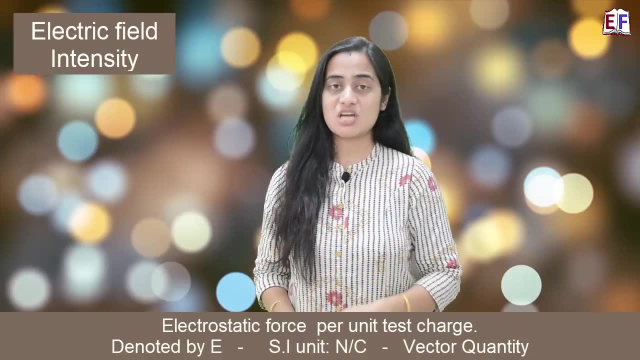 looking at the field lines. so if we are talking about non-uniform electric field lines, looking at which you can tell a lot of things about the electric field, third character's time has come and that is electric field intensity. so what is electric field intensity? it is electrostatic force experienced per unit test charge. 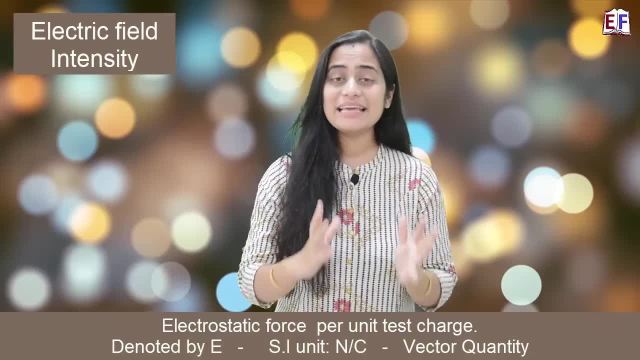 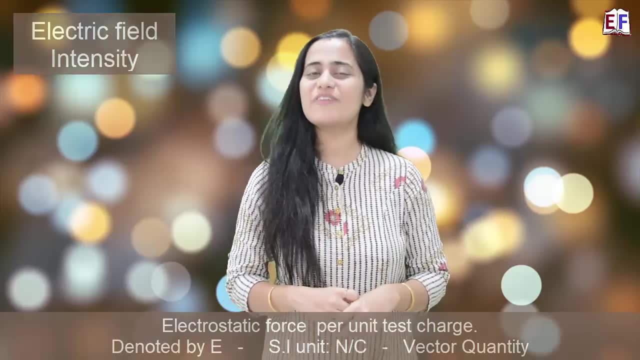 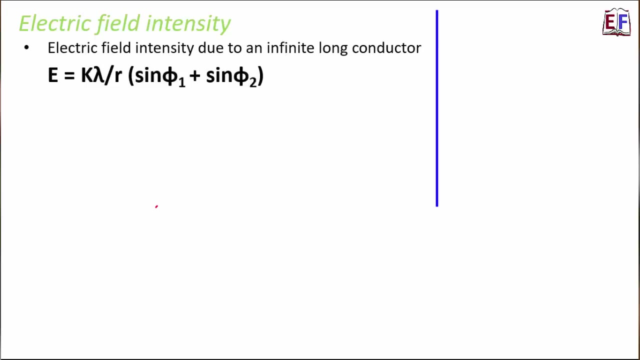 we generally denote it by capital e and E is equal to F by Q. the SI unit for electric field intensity is Newton per coulomb and it is a vector quantity. electric field intensity, every unit is a vector quantity. field intensity due to an infinite long conductor is given by this expression: e is equal to k lambda. 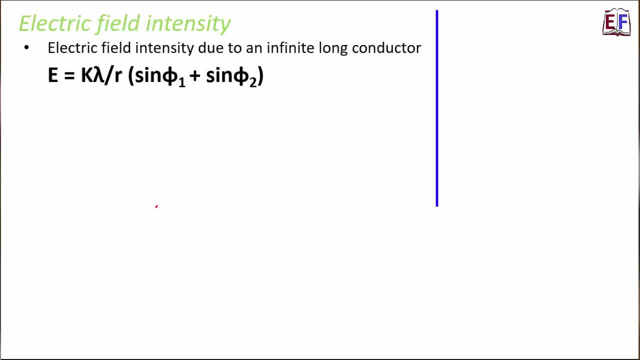 by r sine phi 1 plus sine phi 2. now let us suppose this is an infinite long conductor and we have to find out the electric field intensity at this point: p, which is at a distance, r, then this is the formula that we used. now let me tell you that this is a generic formula for any straight long. 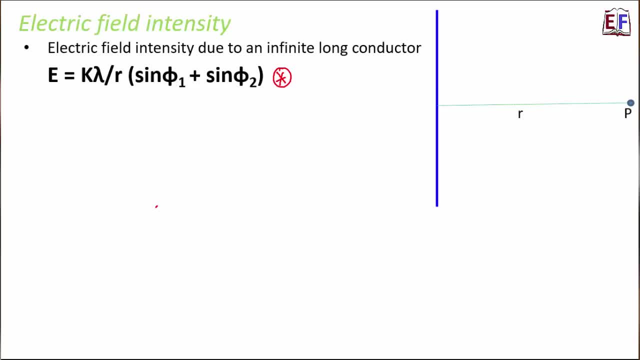 conductor. now, if that conductor is infinite, then what happens? the value of these angles? so these angles are phi 1 and phi 2. so if it is a finite conductor, then we will have some values for phi 1 and phi 2 and we will put them here. but if it is an infinite conductor, that means this is going to 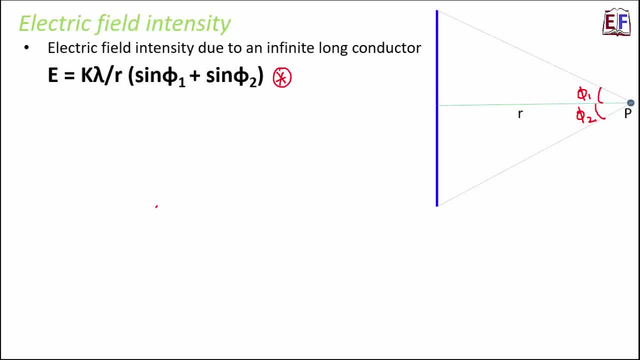 be till infinity. so the values of phi 1 and phi 2 will be equal to 90 degree. so when we put 90 degree then we get the actual expression of the electric field intensity, which is equal to k lambda by r sine phi 1 plus sine phi 2. 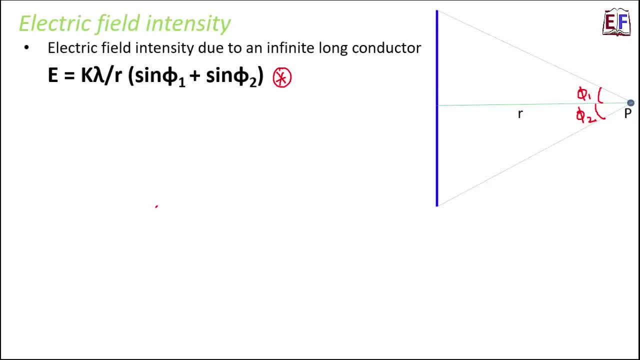 for electric field intensity at point p due to infinite long conductor. now i am not getting into the derivation for these, because that they have already been covered in the detailed version of these videos, so here we are just going to do a crash course on the concepts. the next thing that 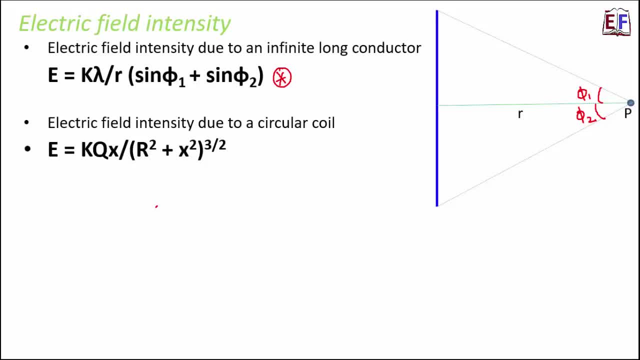 we'll talk about is electric field intensity due to a circular coil. so, and the generic expression is: e is equal to k, q, x divided by r square plus x square to the power 3 by 2. let us suppose this is the circular coil, and this is the point where we want to find. 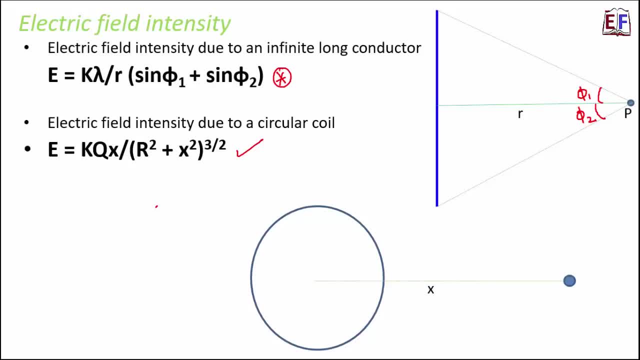 out the electric field intensity. and this point is located at a distance x from the center of the circular coil and r is the radius of this coil. so in this case there could be few special cases. for example, a case one could be: x is very, very greater than r. that means the distance of this. 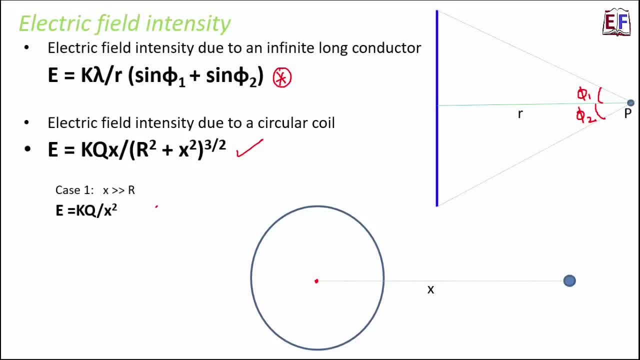 point is very large when compared to the radius of the circular coil. so in this case there could be very few areas where we can actually find out the electrical field intensity, which are extremely high, até if we consider the price of this circular coil. so in that case e becomes equal to kq divided by x square. second scenario could be if the circular 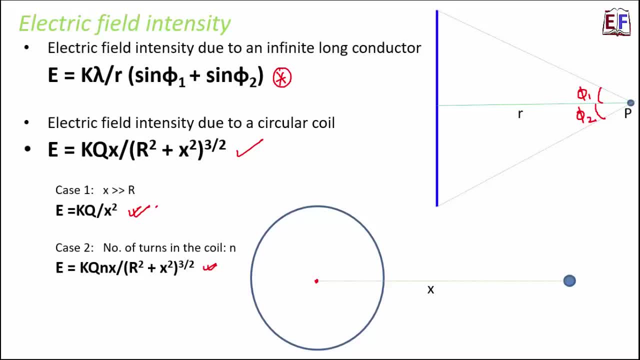 coil has n number of turns. in that case this entire value of electric field also gets multiplied by n. third scenario could be if x is equal to zero. that means what if we want to find out the electric field intensity at the comparison of the electric field at the center of this circular coil? so electric field intensity at the你可以 estimate is 0. 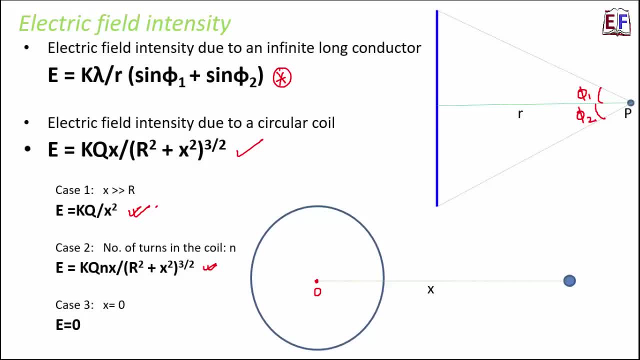 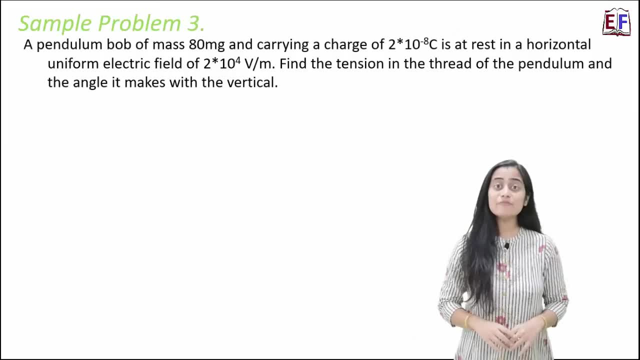 at the center will be equal to zero, because in that case this value of x will be zero, right? therefore electric field intensity will also be equal to zero. it's time for a numerical problem. so here's sample problem three: a pendulum bob of mass 80 milligram and carrying a charge of 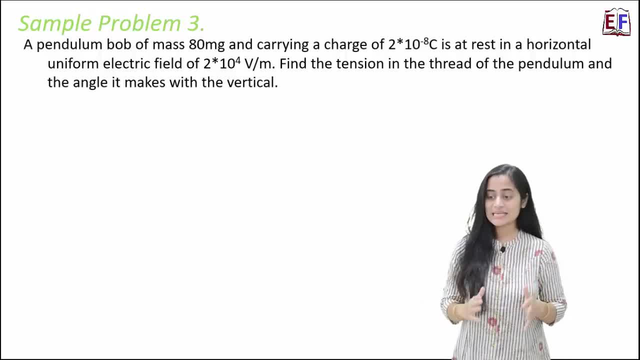 2 into 10 to the power minus 8. coulomb is at rest in a horizontal, uniform electric field of 2 into 10 to the power 4 volt per meter. find the tension in the thread of the pendulum and the angle it. 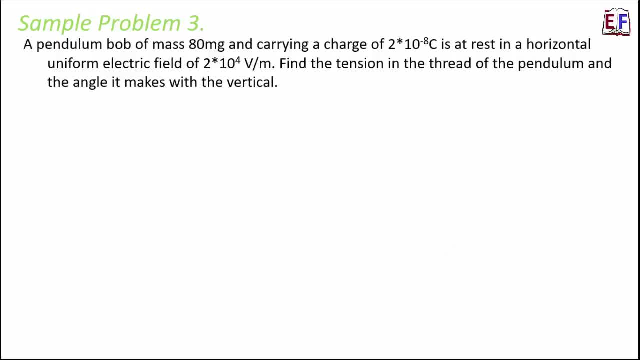 makes with the vertical. as always, let us first note down what are the values that are given to us. so mass is given as 80 mg, 80 milligram, that is, 80 into 10, to the power minus 6 kgs. okay, charge, that is. q is given as 2 into 10 to the power minus 8 coulombs, and electric field e. is given as 2 into 10 to the power minus 8 coulombs, and electric field e is given as 2 into 10 to the power minus 8 coulombs, and electric field e is given as 2 into 10 to the power minus. 10 to the power minus 8 coulombs, and electric field e is given as 2 into 10 to the power minus 8 coulombs, and electric field e is given as 2 into 10 to the power minus 8 coulombs. 10 to the power, 4 volt per meter. 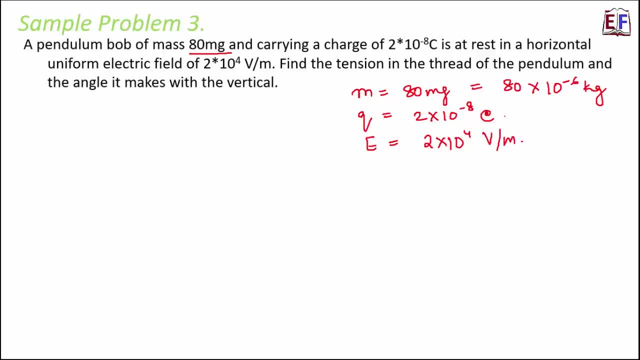 okay, now let us try to draw a rough diagram of the scenario. so this says that this is a pendulum with a bob of mass, 80 milligram. right, so this is at rest in a horizontal uniform electric field of 2 into 10 to the power, 4 volt per meter. so now, as the pendulum moves like this, so it makes some 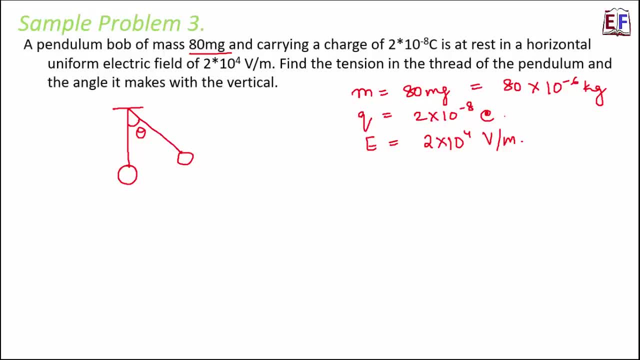 angle theta with the vertical right, and that angle theta is what we need to calculate in this question. so let us draw a free body diagram of the bob of this pendulum. so mg will act in the downward direction, as always. so this is tension t, so this angle is also theta. 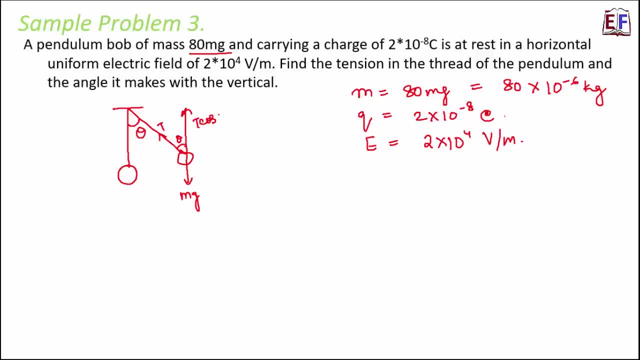 because this is theta, this is also theta, so this becomes t cos theta. this side will be t sine theta. and what will be this side, this side? it will experience an electrostatic force. and this electrostatic force is how much this is q into e. so that's the relationship between. 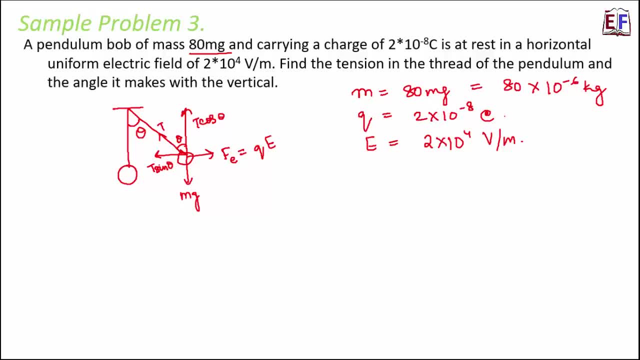 electrostatic force. and now what happens at equilibrium? so all these forces need to balance, correct. so therefore, t cos theta needs to balance mg and t sine theta needs to balance q e. now let us divide these two equations, or what we can do is let's say: this is one, this is two. so if we do, 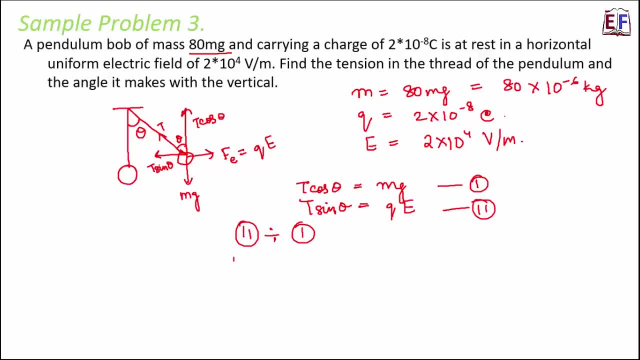 two divided by one, then what happens? we get tan. theta is equal to q. e divided by mg. so therefore now let us calculate this. so q is given as 2 into 10 to the power minus 8, e is 2 into 10 to the power 4 divided by m is 18 to 10 to the power minus 6 and g is 9.8 mean. 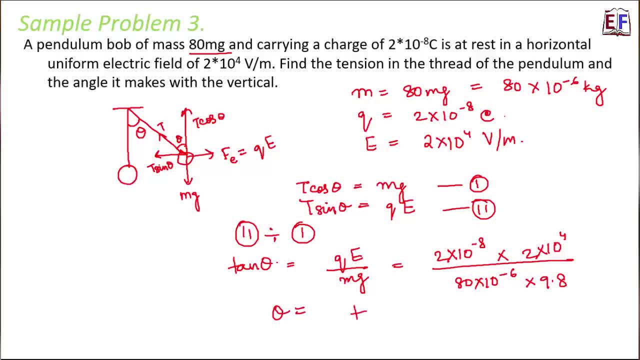 per second square. so theta becomes equal to tan. inverse this entire thing. when we calculate it comes out to be 0.51. so therefore theta is equal to 27 degrees. so that's the angle that it makes with the vertical. but we also need to calculate the tension. but i think that we can very easily. 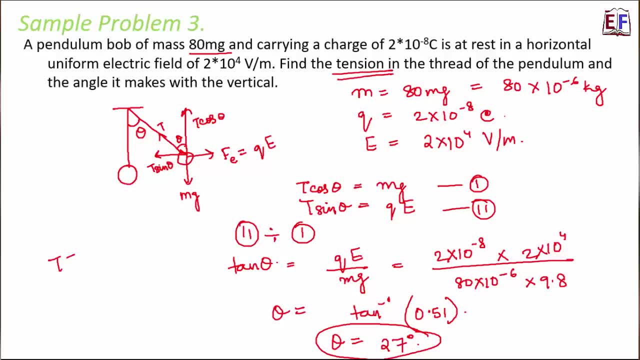 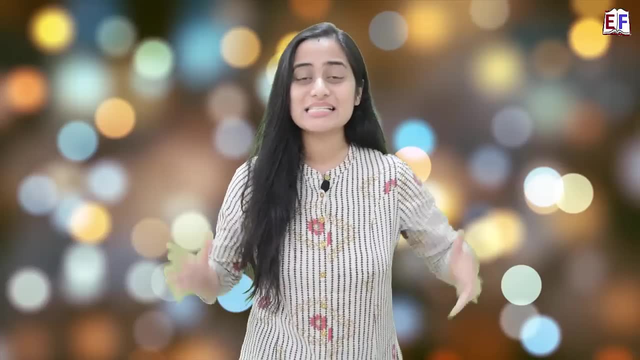 calculate now, because from equation 1 we see that t is equal to mg by cos theta. so mg we already knew and theta also we know now, so we can easily calculate tension. The next character's entry time is up and the next character we are going to introduce is electric dipole. yes, very, very. 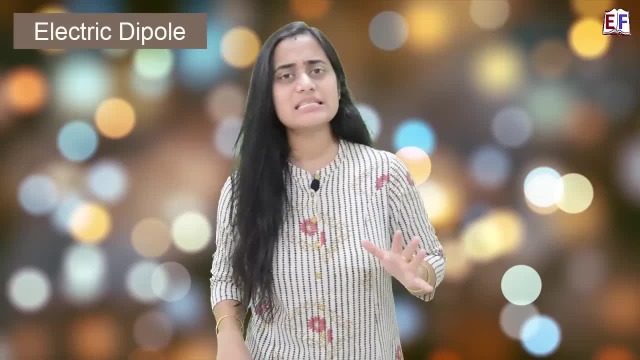 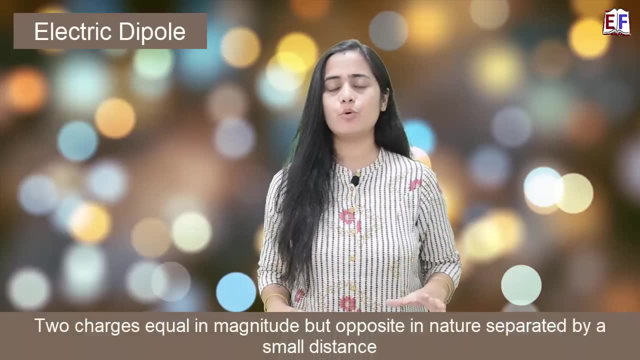 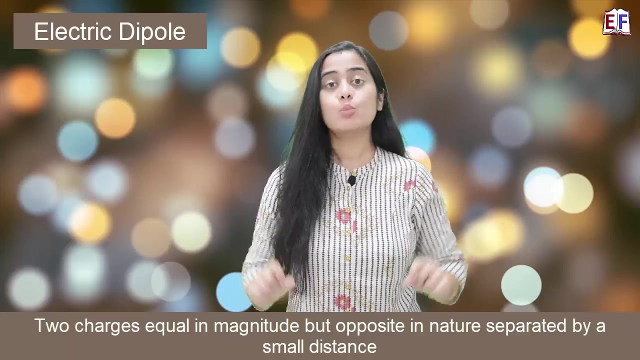 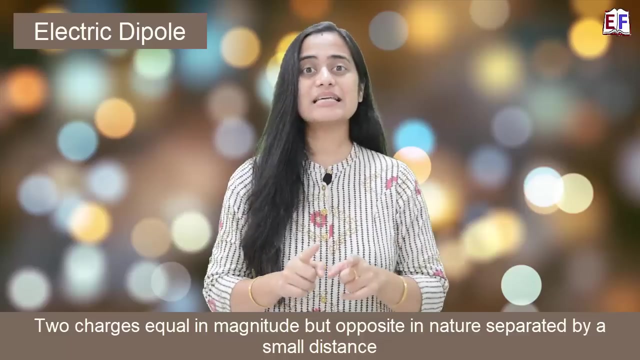 important questions come. you must understand very conceptual. you get numericals, you also get derivations. so let's focus. what is electric dipole? di means two. so here we are talking about two charges which are equal in magnitude but opposite in nature, separated by a small distance. that is electric dipole. so if one charge is plus Q, the other is minus Q. 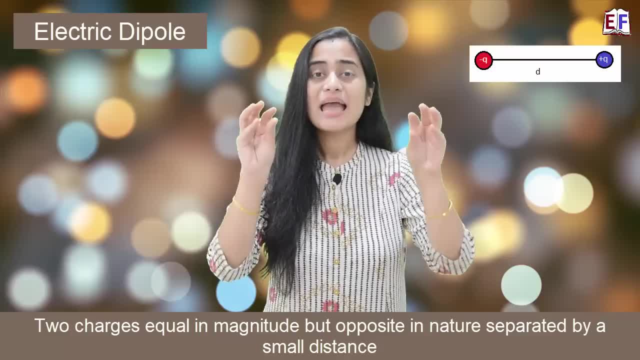 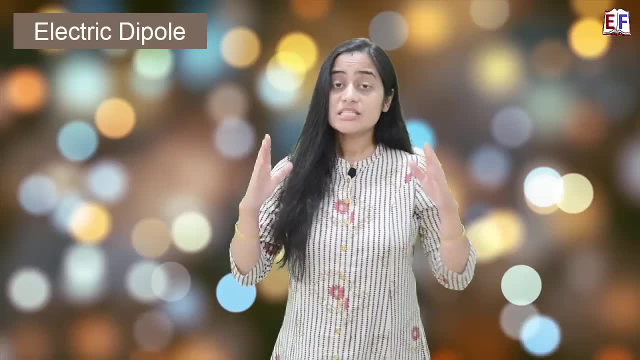 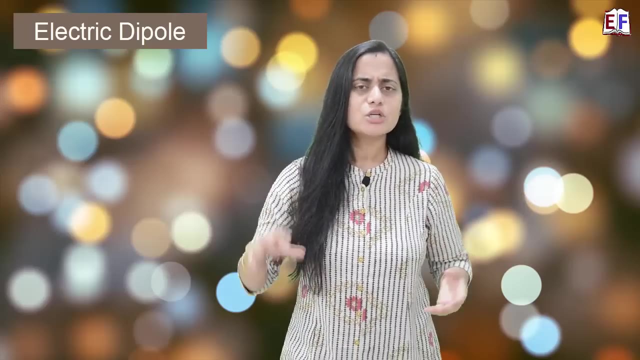 if one is plus 2 Q, the other is minus 2 Q. such two equal and opposite charges, separated by a small distance, is called electric dipole. where we will talk about electric dipole, we will talk about dipole moment. what is dipole moment? so dipole moment basically talks about the strength of 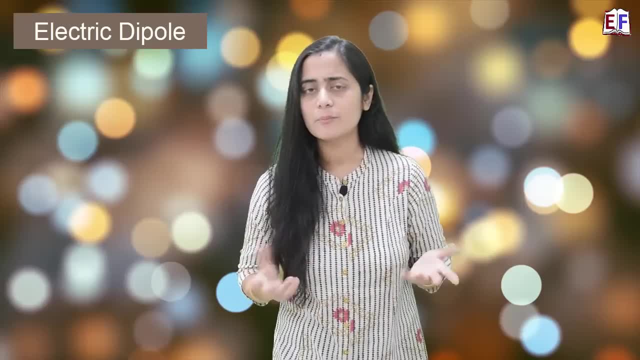 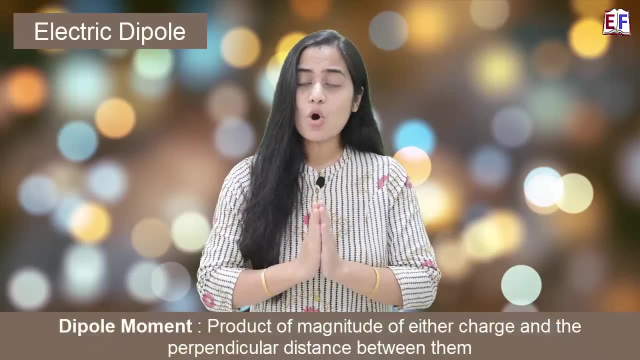 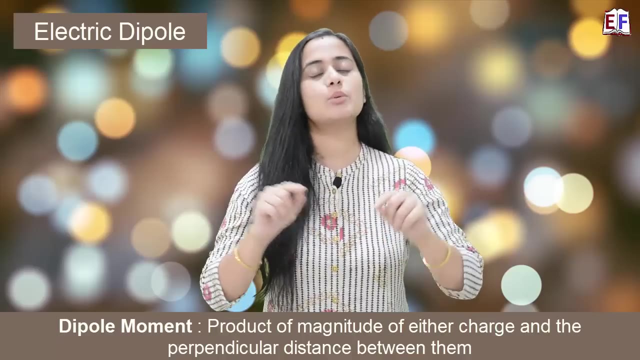 the electric dipole, how strong is the dipole, how weak is the dipole? that that comes out from dipole moment. now how do we calculate dipole moment, product of the charge and the distance between the two charges, basically the perpendicular distance between the two charges. so that gives us dipole moment, the unit for 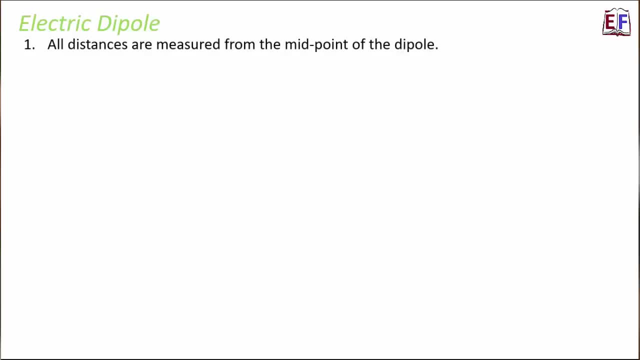 dipole moment is Newton Coulomb and it is a vector quantity. few important things about dipole moment. dipole moment is a vector quantity. important points to remember while we deal with electric dipoles. all distances are measured from the midpoint of the dipole. so, for example, let us suppose we have a dipole say minus q and plus q. 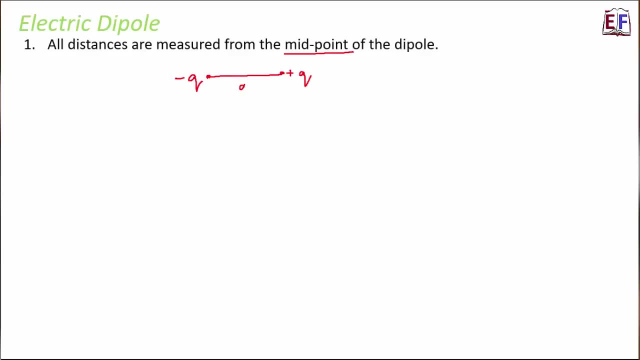 which is separated by distance, say d. so in that case, if i am talking about some random point, if i am talking about any measurements from the dipole, i say that there is a point p which is located at a distance x from the dipole. that means this x will be measured from the midpoint of the 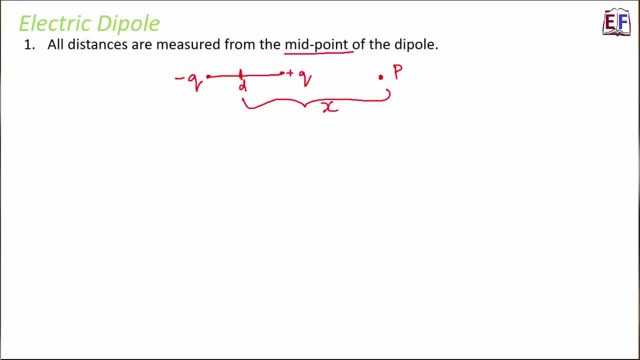 dipole, so any measurement has to happen from the midpoint of the dipole. second thing: ideal dipole. you will come across this word, ideal dipole, sometimes. and what does that mean? it means that the charges are of large magnitude and they are separated by very small distance. that means 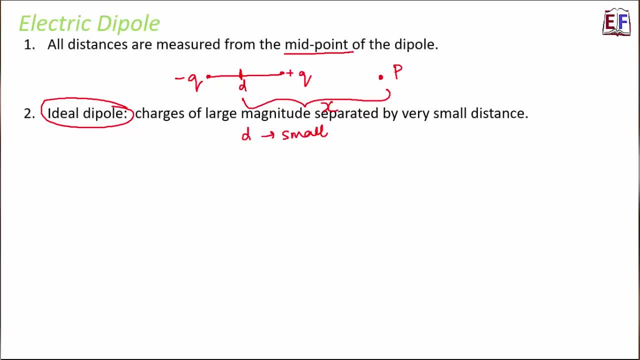 d is very small, whereas the magnification of the charge is very large. so big charges separated by small distance, that's an ideal dipole. another term that you will come across is quadrupole. the word quad quadru means four. so when we deal with four charges- because in a dipole normally we have two charges- 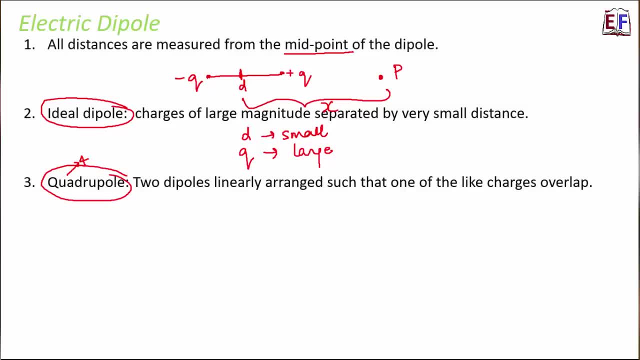 but when we deal with two dipoles which are linearly arranged such that one of the like charges overlap, that is called a quadrupole. now, in quadrupole also, we have two types of quadrupole. one is a positive quadrupole, which is somewhat like this: this is called a positive quadrupole. 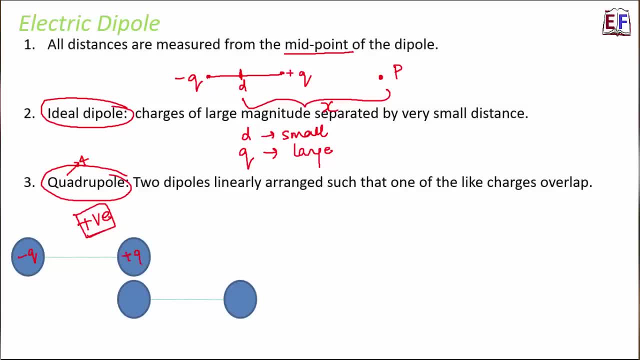 here what happens is, let's say, this is minus q, this is plus q, this is plus q, this is minus q. so what happens? two positive charges of the two dipoles they are, they overlap, so this is a positive quadrupole. so can you guess what would be a negative quadrupole? obviously the negative. 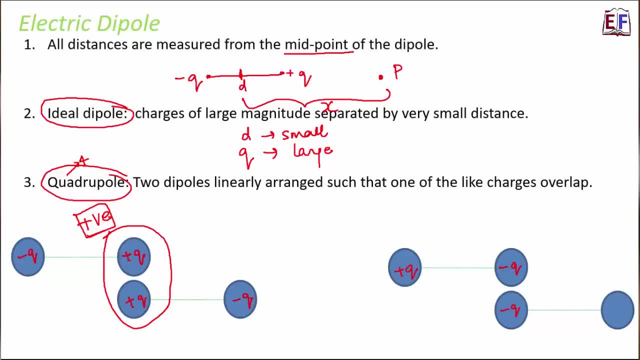 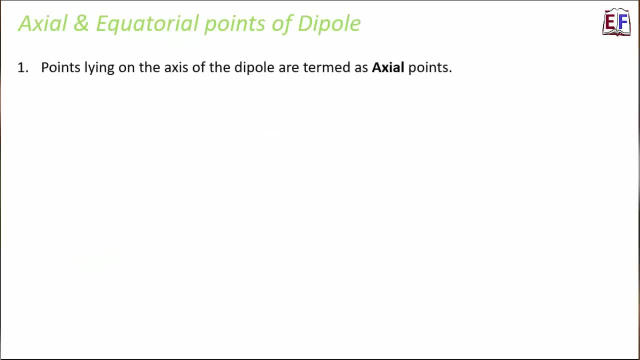 charges would overlap in this case and the positive would be on the two ends you. so this one is a negative quadrupole. very important topic: axial and equatorial points of dipole. so axial point, the name itself says that it has something to do with the axis. so points lying on 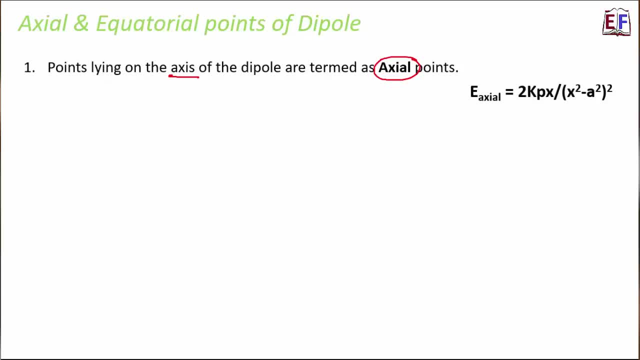 the axis of the dipole. so let's say: if this is the dipole. so let's say: if this is the dipole, let's say this is minus q, this is plus q, and they are separated by a distance: 2a. so why it is 2a? because you know that makes the calculation and the derivations little easy. 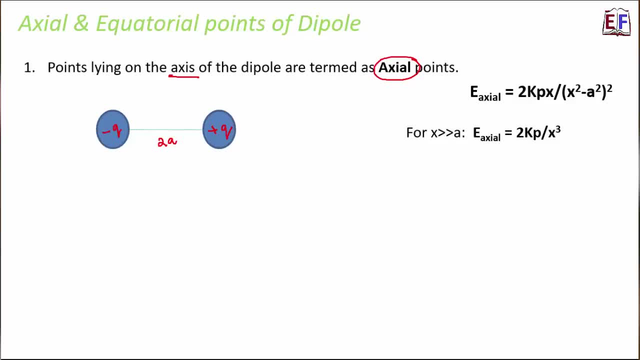 so we take that as a convention, that the distance between the dipole, between the two charges of the dipole, is 2a. so how do we calculate the electric field at an axial point of the dipole? so let us suppose that if this is a point p which is lying on the axis, therefore axial point. 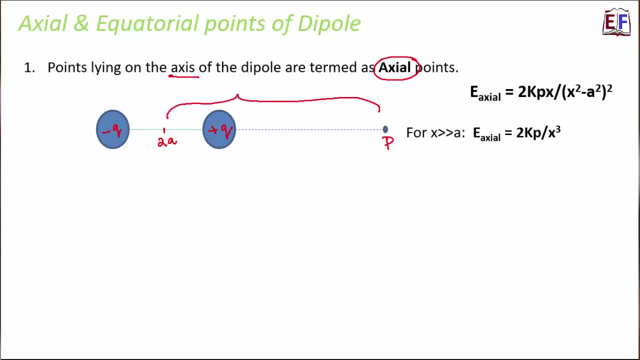 and it is at a distance x from the midpoint of the dipole. So what would be the electric field at this point? So electric field is given by 2kpx divided by x square minus a square, whole square, and for x very, very greater than a, as in if this point is located very far away, in that case, 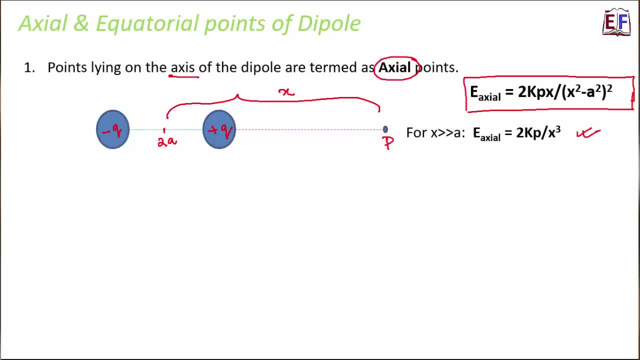 it is given by 2kp divided by x's cube. Again, I am not getting into the derivation in this video, this being a crash course. however, for detailed derivation please refer to the link in the given in the description section. Now let's talk about the equatorial points. 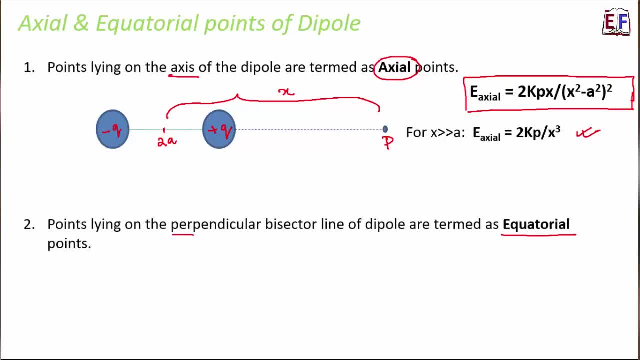 So equatorial points are those which are lying on the perpendicular bisector line of dipole. So, for example, this is how we calculate the electric field at an equatorial point. So if this is a dipole, this is the perpendicular bisector. so any point lying here, for example, 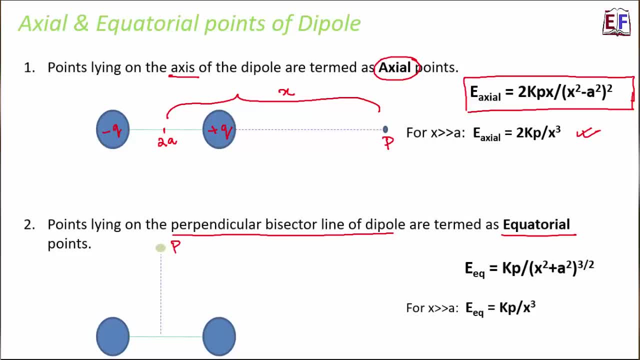 if this is the point P, which is an equatorial point. So electric field at this point is given by kp divided by x square plus a square to the power 3 by 2.. Again, for x, very, very greater than a e, equatorial is kp by x's cube. 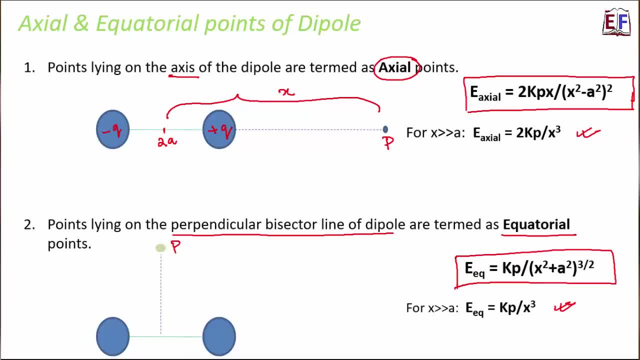 So if you compare these two, you see that for points which are very far away from the midpoint of the dipole, e axial is 2 times e equatorial. Let us see what happens to a dipole placed in an uniform electric field. Well, 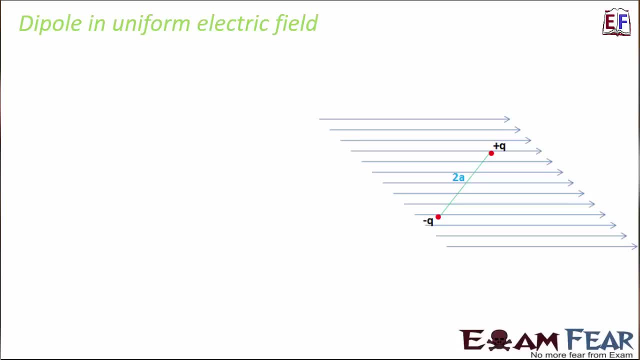 When a dipole is placed in an uniform external electric field, it experiences what we call as torque. and why does it experience torque? that's because, let us suppose, if this is a dipole minus q, plus q separated by 2a, right, Let us call this point as a. let us call this point as b, just for the convenience to explain. 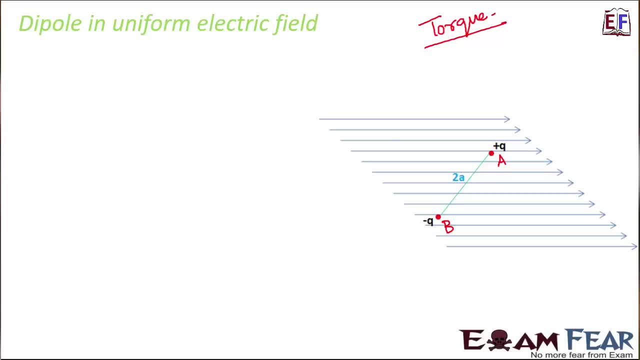 Now, force at point a would be qe. So the force at this point will be equal to qe, And the force At this point, magnitude wise, will be equal to qe, but in the opposite direction, Right. So here the force would be in the direction of the electric field, that is, this direction. 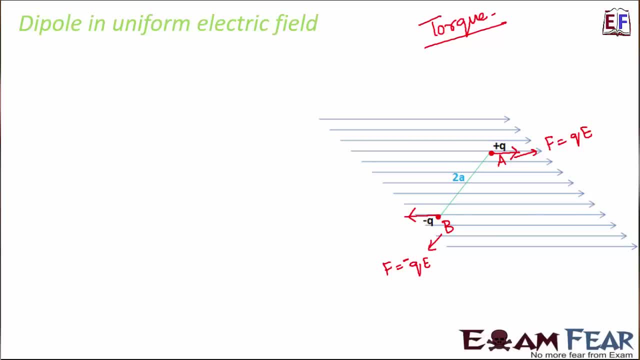 here it will be opposite direction. Now, what happens now? even though the net translatory force is 0, because magnitude of the forces are equal and they are opposite in direction, But since their line of action is not same, So what happens here? This force will try to push it in this direction. this force will try to push it in this direction. 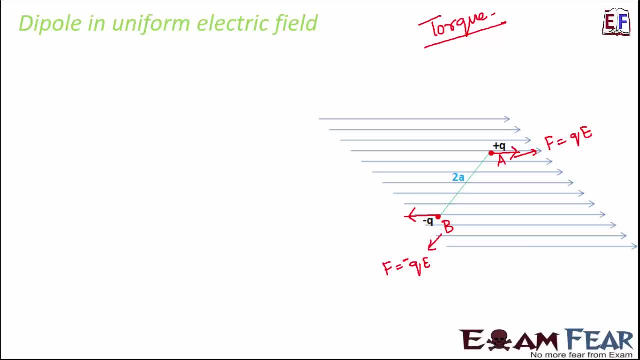 and as a result this entire dipole or this entire rod will start rotating. so, and that is what is called as torque. So here net force is equal to 0, but net torque is non-zero. So how much is the torque experienced by this dipole? torque is given by p cross e, where 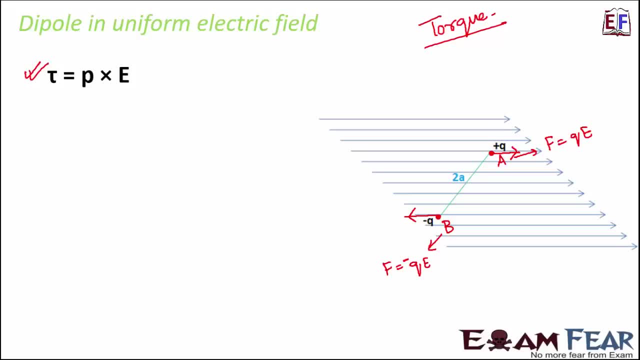 p is the dipole moment and e is this electric field. So p cross e, E is basically p e sine theta, where theta is the angle that it makes with the electric field. Now, when is the torque maximum? when the value of sine theta is maximum. 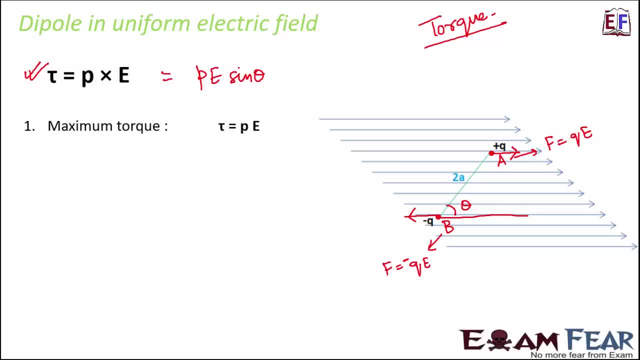 So maximum value of sine theta is when theta is 90 degree, sine theta is 1.. So maximum torque is p? e. When is the torque minimum? when sine theta is minimum. minimum value for sine theta is 0.. So minimum torque is 0.. 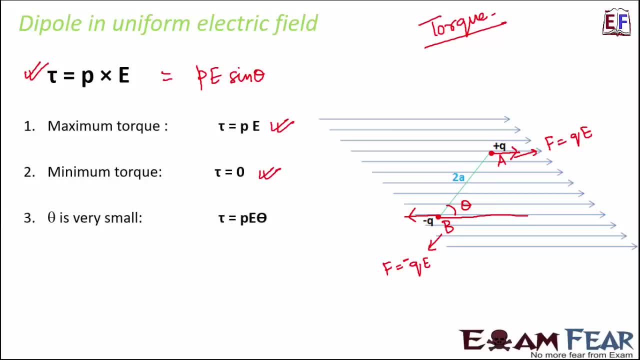 When the value of theta is very small, then sine theta can be approximated to theta. So in that case torque will be equal to p e. theta Time period is given by 2, pi. root over i by p e, where i is the moment of inertia. 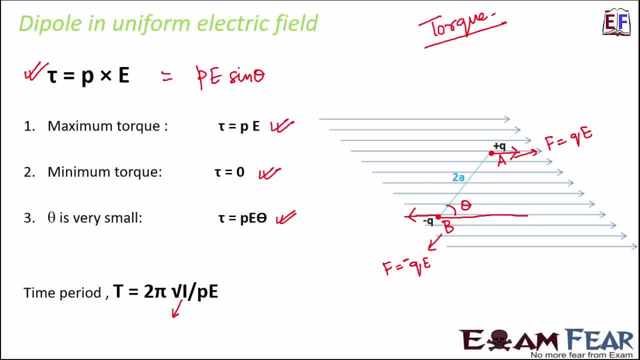 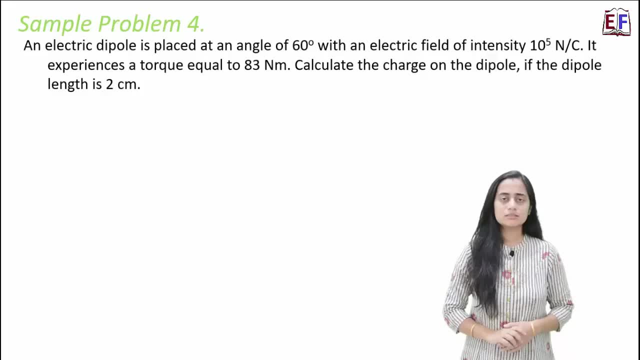 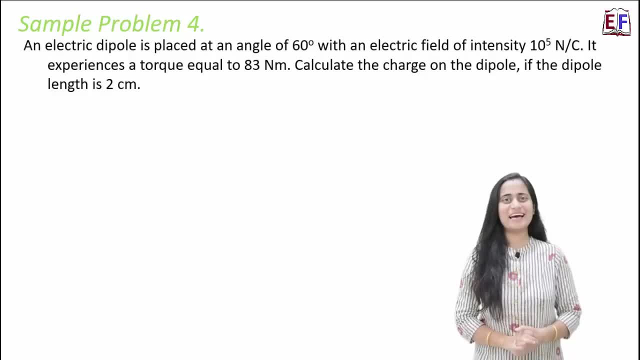 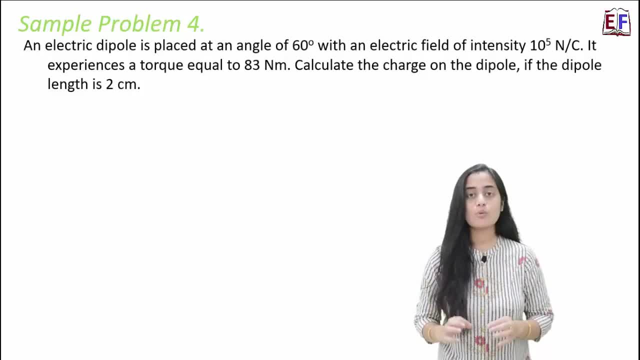 with an electric field of intensity 10 to the power, 5 newton per coulomb, It experiences a torque equal to 8 root over 3 newton meter. Calculate the charge on the dipole if the dipole length is 2 centimeters. 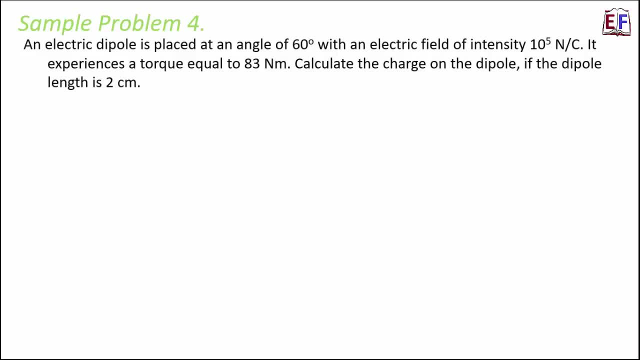 Please note down, as always, what are the values that are given to the dipole. Please note down, as always, what are the values that are given to the dipole. Electric field is given as 10 to the power 5 newton per coulomb. theta is given as 60 degree. 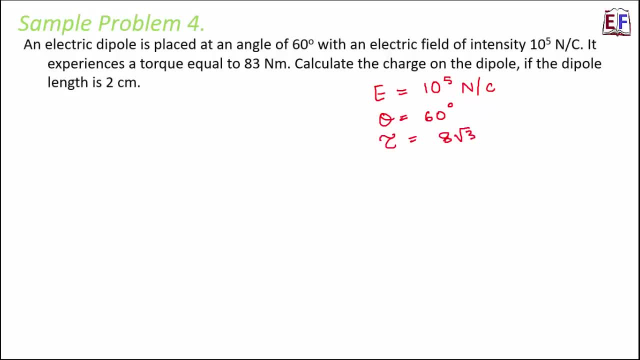 torque is given as 8 root, 3 newton meter, and we have to find out the charge on the dipole. So how do we calculate torque? torque is given by P cross E. that is equal to P E sine theta. So from here we can say that Q. 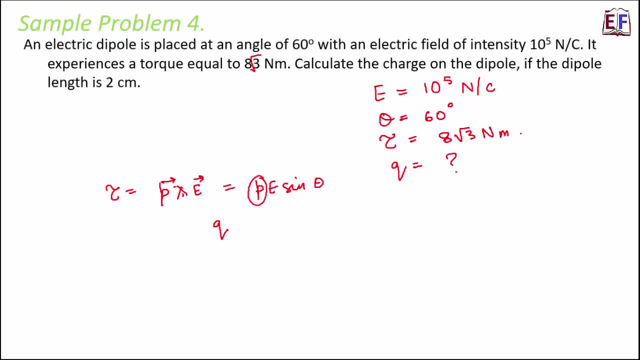 And what is P? p? p is basically the product of the charge multiplied by the distance between the dipole. so if the distance we assume to be d, so in that case torque is equal to q, d e sine theta. so q is equal to torque divided by d e sine theta. so let's put the values. so torque is given as 8 root. 3. 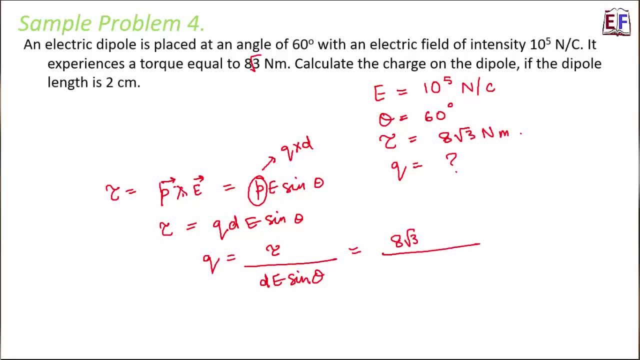 divided by d, that is the length of the dipole, which is 2 centimeters. so this is 2 into 10 to the power minus 2 meters. into e is given as 10 to the power 5 sine theta is sine 60 degree. 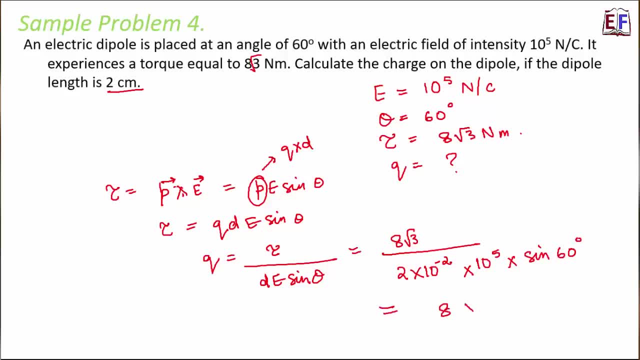 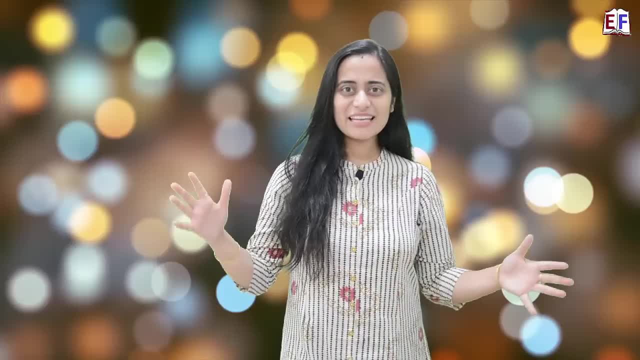 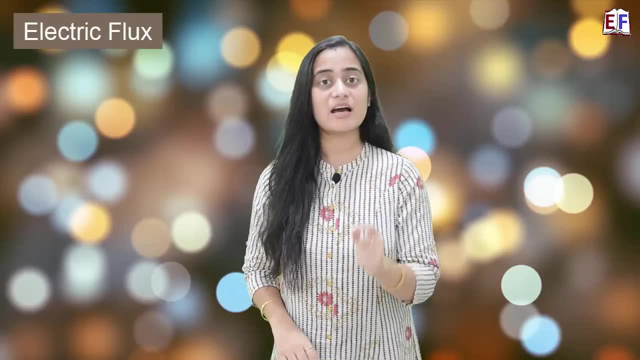 so when you calculate this, it comes out to be 8 into 10 to the power minus 3 coulomb. so that's the charge on the dipole. finally, the last character of the movie is electric flux. yes, So what is electric flux? Electric flux tells us the number of electric field lines crossing per. 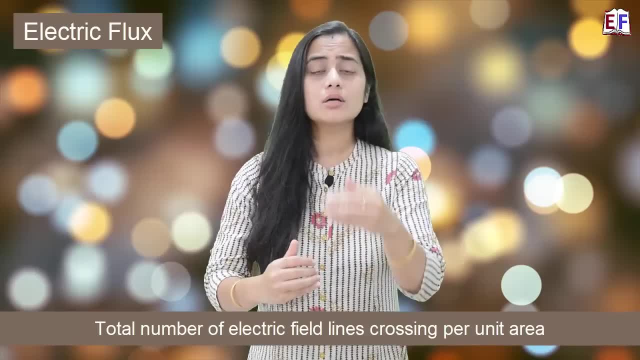 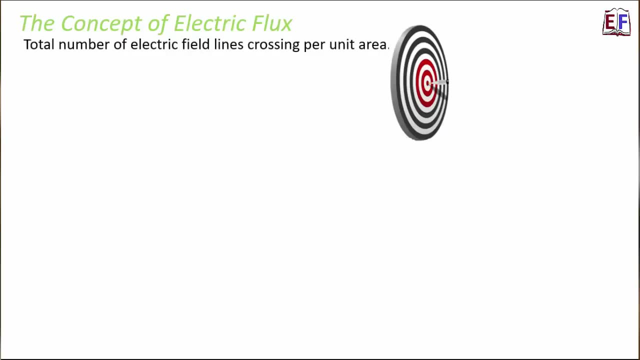 unit area. but there is a lot more to electric flux. Let us take the example of this dart board here to understand the concept of electric flux. So what do we see? In the first case? this is the board and this is how the arrows hit the board. So what do we see? We see that most of the arrows 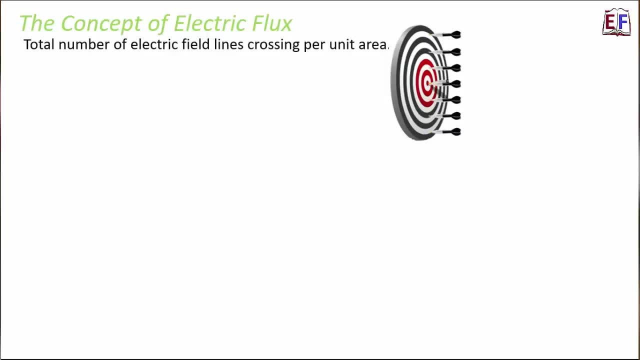 they like they strike the board. Now I keep the same board as in. the area of the board remains the same, but I just change the orientation of the board. What happens? Do we still have the same number of arrows hitting the board? No, not really. So now those many arrows are not hitting. 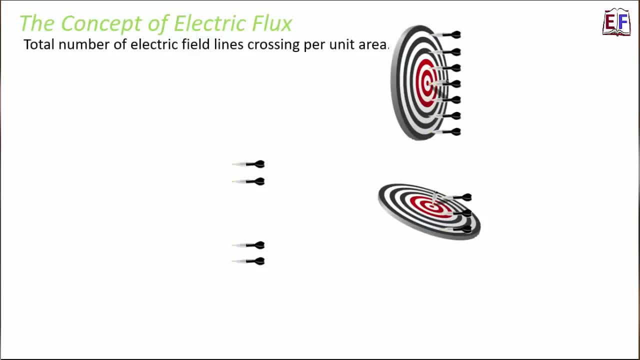 the board. A lot of them are passing through it. Now I further change the orientation of the board and what happens? We see that all the arrows are passing through the board. So that means here it is not just the area of the board that matters, but also. 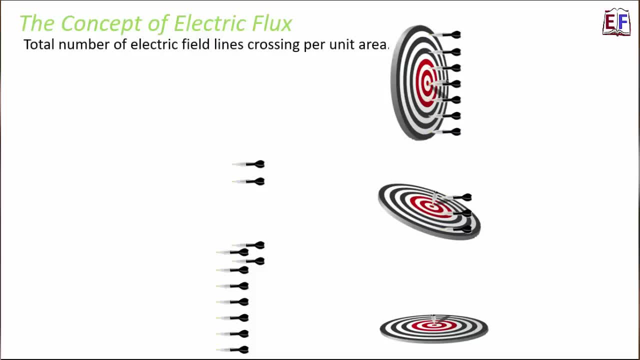 the alignment or the orientation of the board. that also matters In a very similar way when I talk about number of electric field lines. these electric field lines are like these arrows, So how many lines will pass through a particular area not only depends on the magnitude of the area, but also on 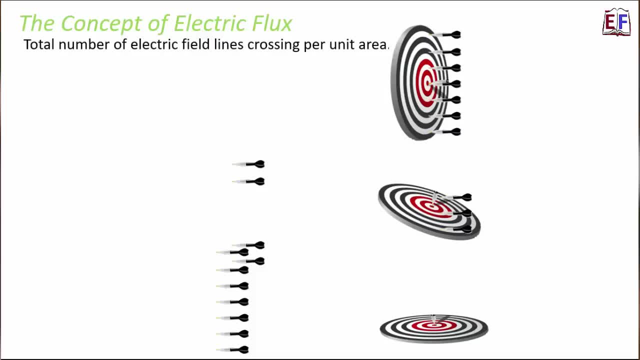 the orientation of the board. So what do we see? In the first case, this is the number of arrows hitting the board. What happens? Do we still have the same number of arrows hitting the board? No, not really. So direction or orientation of the area also matters, and that is why we talk about area vector when we 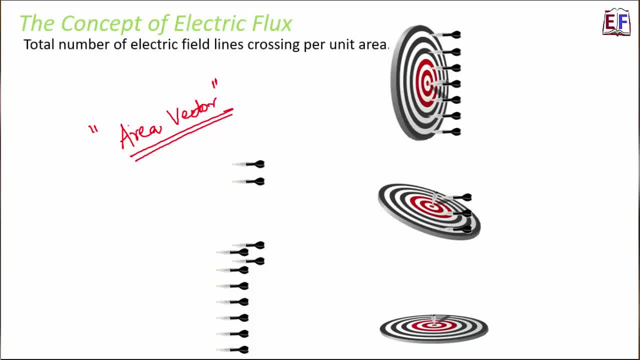 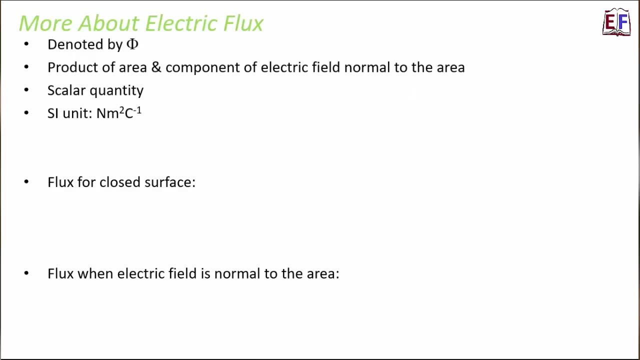 talk about the concept of electric flux. We just do not talk about area, We talk about area vector and you will see that a theta get involved and that theta tells us what is the orientation of the area vector, A few important things to know about the area vector. So the area vector is a 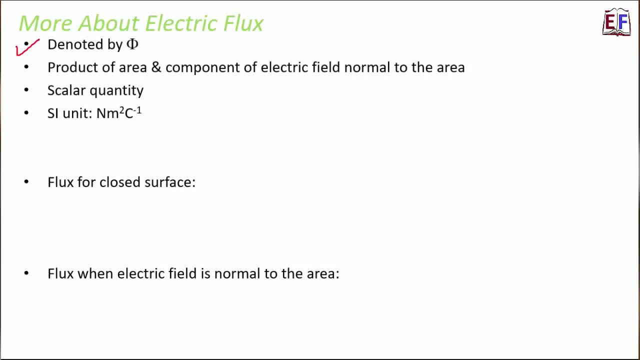 slope vector. essentially, That is what we are going to recall later on. We are also going to discuss a little bit about the electric flux already. Now, let is me say: okay, now let us talk about electric flux. It is denoted by phi. It is product of. 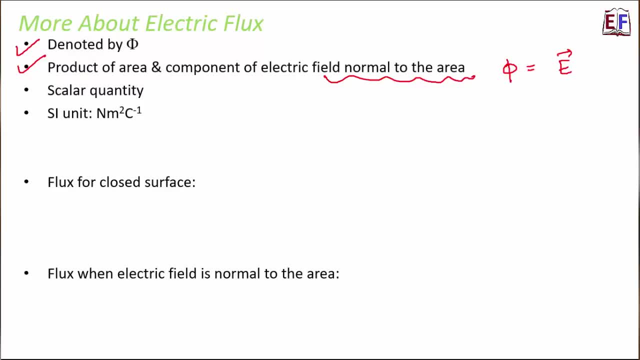 area and component of electric field normal to the area. So this component thing takes care of the orientation of the area with respect to the electric field. So how do we denote it? So phi is equal to with respect to the electric field. it is a scalar quantity. si unit is newton meter square per coulomb. 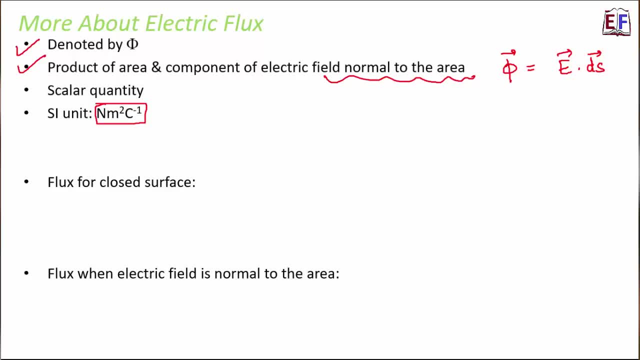 that's quite obvious, because it is a product of electric field and area flux for closed surface. how do we denote the flux for a closed surface? e dot ds for a closed surface. this is how we denote it- flux when electric field is normal to the area. now phi is equal to e dot ds, which is equal to e. 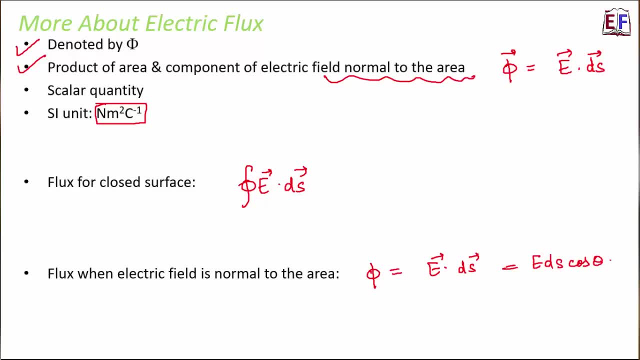 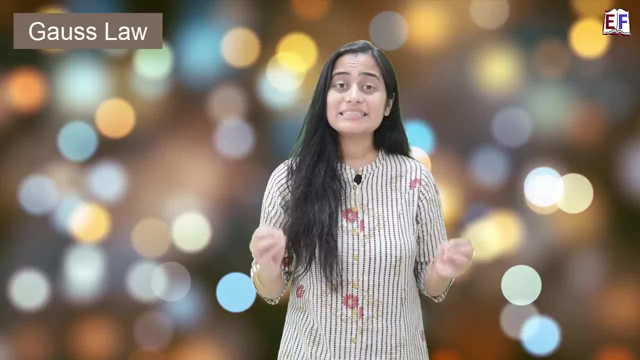 ds, cos theta now, when electric field is normal to the area. so theta is 90 degree cos theta is zero. therefore phi is equal to zero, so flux is equal to zero. gauss law- a very important topic, a very important law exams. may kai baar gauss law. 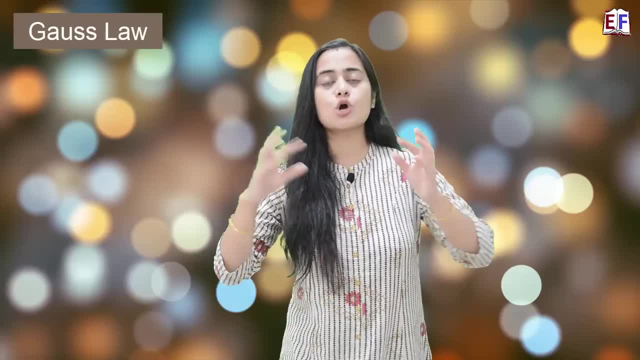 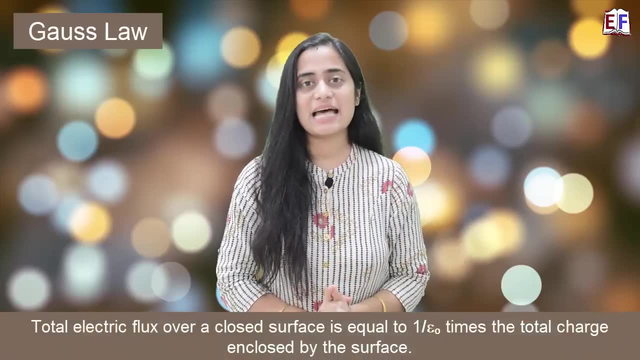 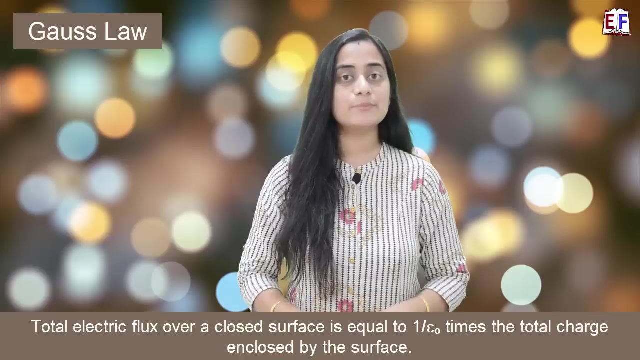 prove karne bola jata hai. kai baar bola jata hai. using gauss law. derive this prove that. so gauss law overall is very important. and what is gauss law? so gauss law states that the total electric flux over a closed surface is equal to 1 by epsilon naught times the total charged enclosed. 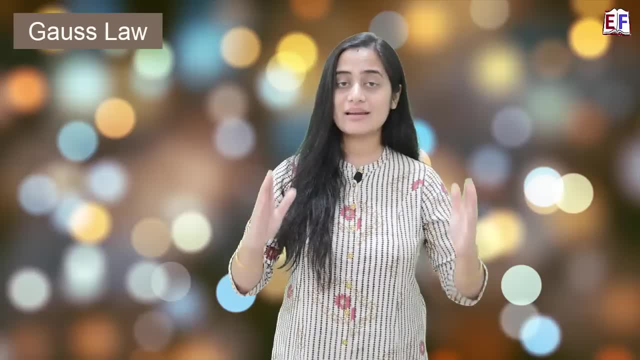 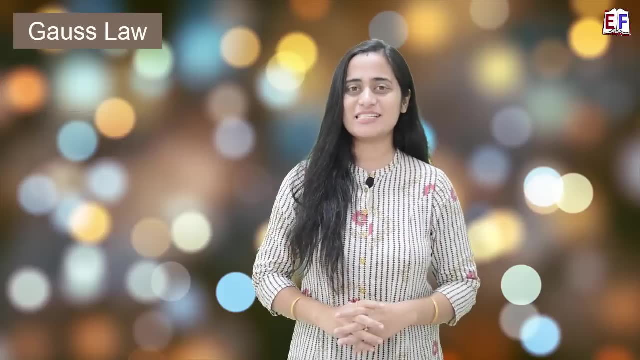 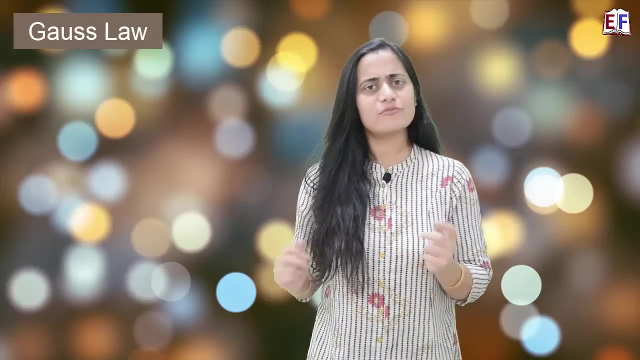 by the surface, that is. in short, we can write: phi, which is electric flux, is equal to q by epsilon. naught for a closed surface. now gauss law is true for any closed surface, yes, for any closed surface. now, why do we have gauss law? because it makes calculation of electrostatic field easier when the system has a symmetry. 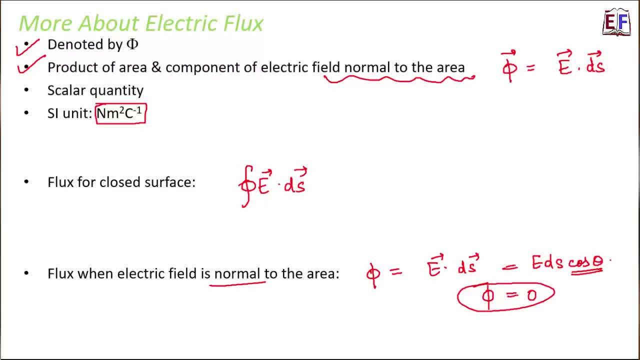 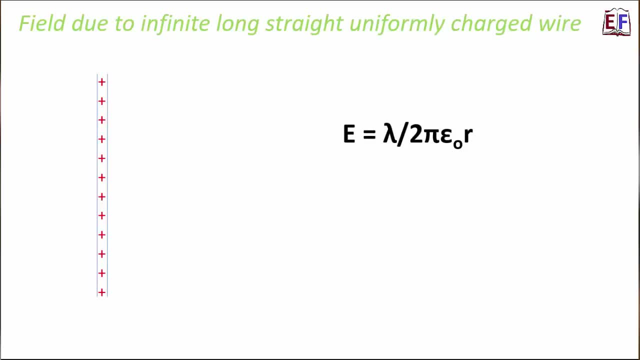 do you want to know how? let's take a look now. this is important from exam perspective. you are often asked to calculate electric field using gauss law. so if you have to calculate field due to infinite long, straight, uniformly charged wire which calculate electric field using gauss law, 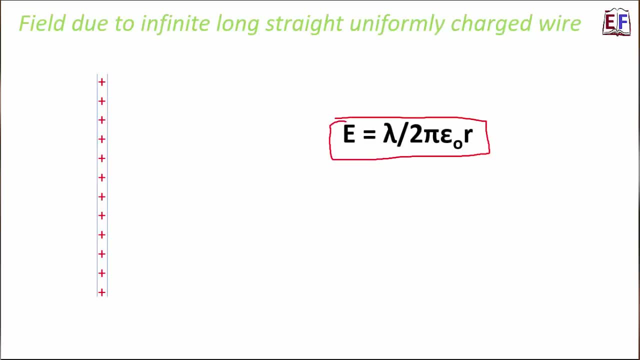 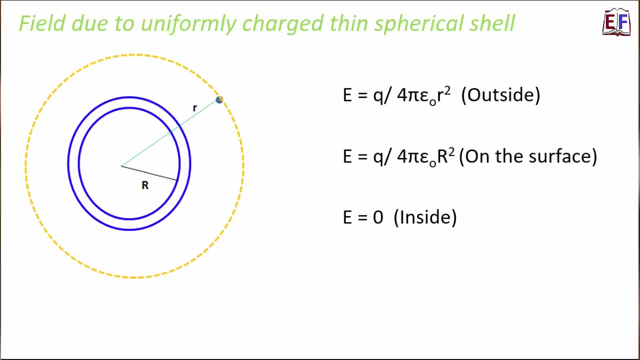 comes out to be lambda, divided by 2, pi, epsilon, naught, r. but in order to get this you need to assume a gaussian surface, which we assume as a cylinder, like this, such that that long straight charged wire passes through the center of this cylinder field due to a uniformly charged thin. 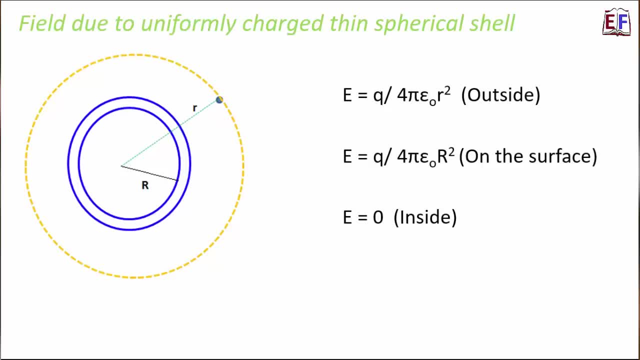 spherical shell. so this blue colored thing that you see, that is the thin spherical shell. now we take a gaussian surface like this, as you can see here. so electric flux is equal to 1 by 2 pi. epsilon naught r square, where r is the distance of the point on the surface, e is equal. 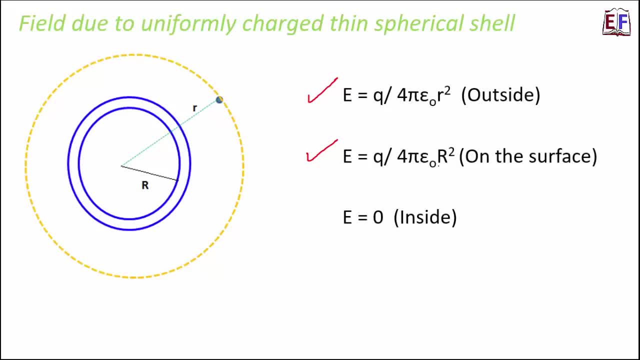 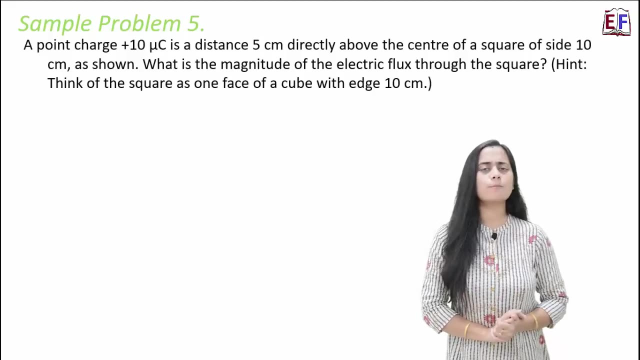 to q by 4 by epsilon naught r square, where capital r is the radius of this spherical shell and electric field inside is equal to 0. again, i am not getting into the derivations. for derivations please refer to the link in the description. finally, the last numerical problem for this lesson, and that is: 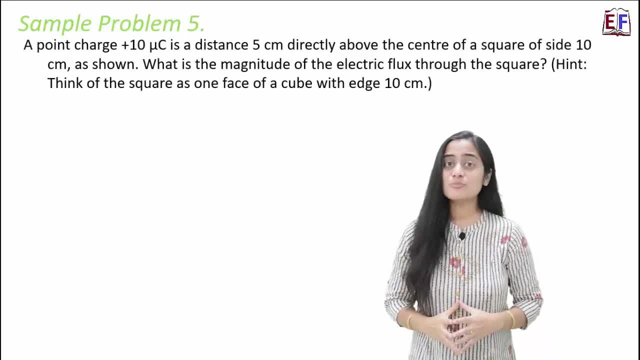 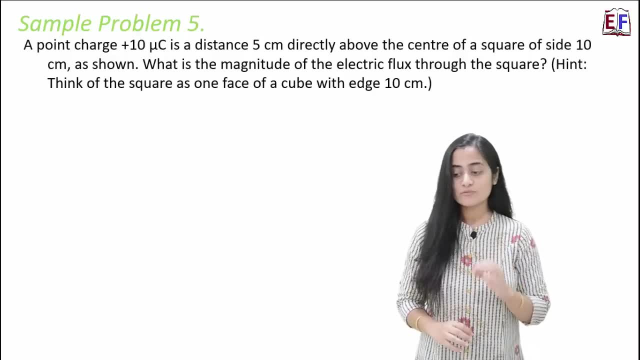 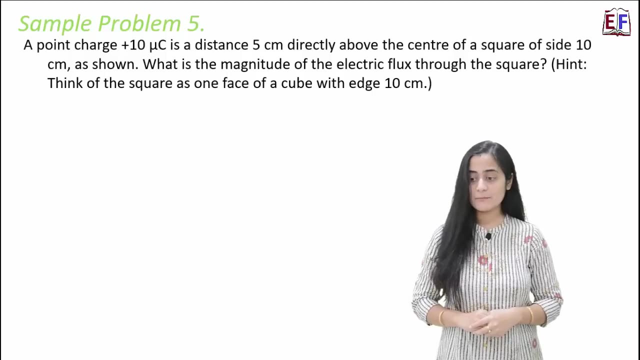 sample problem 5: a point charge of plus 10. micro coulomb is at a distance of 5 centimeter directly above the center of a square of side, 10 centimeter, as shown. what is the magnitude of the electric flux through the square? and there is a hint. think of the square as one face of a cube. 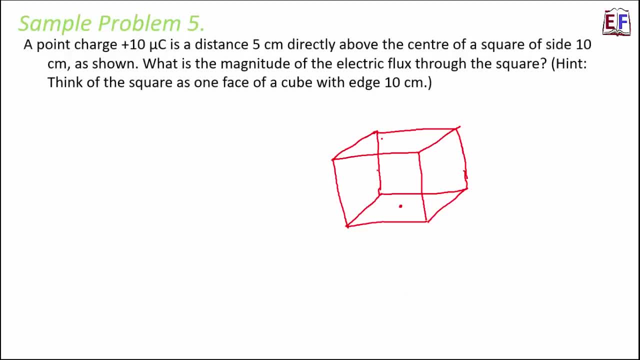 whose edge is 10 centimeters. let's take help of the hint which says that the square is one face of a cube with edge 10 centimeter. so let us suppose that this face is the square that we are talking about. so it says that there is a point charge somewhere here which is at a distance of 5. 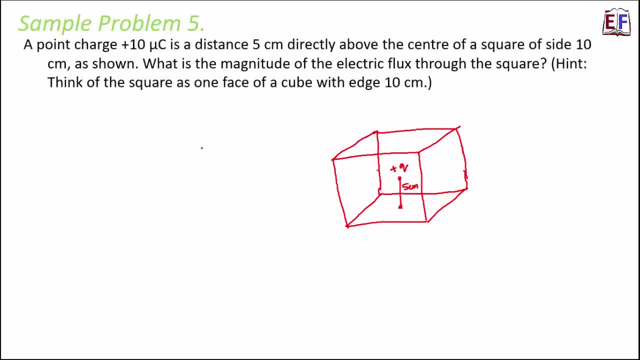 centimeter from the center of the square right- perfect. so now in the question it is given that q is 10 micro coulomb, that is 10 into 10 to the power minus 6 coulomb. we need to find out the value of electric flux now for this entire cube. 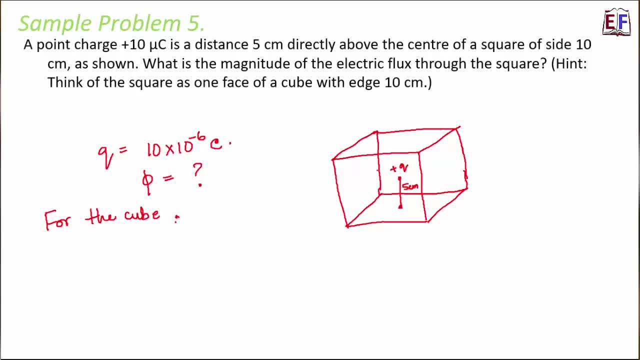 just the square for the entire cube. if we apply the gauss law, we can say that the total Phi will be equal to Q by Epsilon naught right now. one face is a square. now how many faces are there in this cube? there are six faces right, so that means the electric flux through this particular square will. 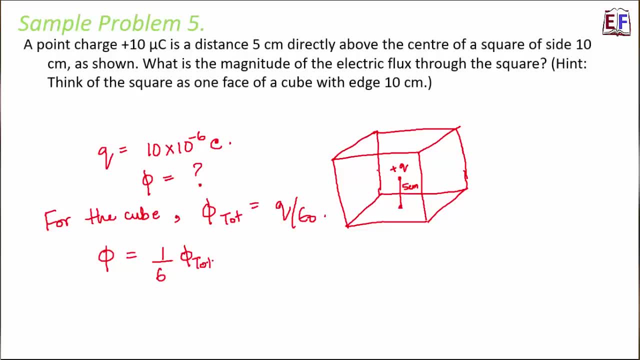 be equal to one sixth of the total electric flux through the cube. that is equal to one by 6 Q divided by epsilon naught. so this will be equal to 1 by 6 into 10 into 10 to the power minus 6 divided by epsilon naught is 8.85 into 10 to the power minus 12. so you: 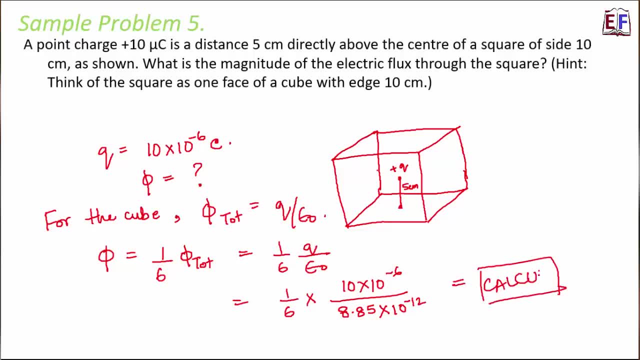 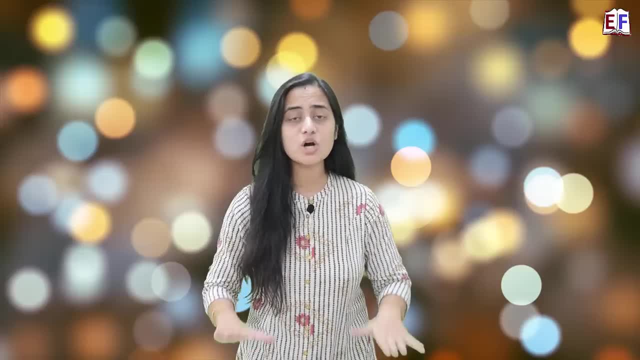 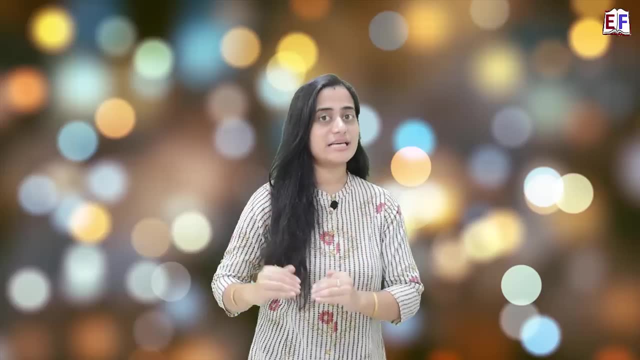 can calculate and get your answer. So that was our crash course on electric charges and fields and we covered all the topics, all the concepts, all the formulae, but with less numericals and without derivations. so for all of those who want to learn the detailed derivations and want to solve more numerical, 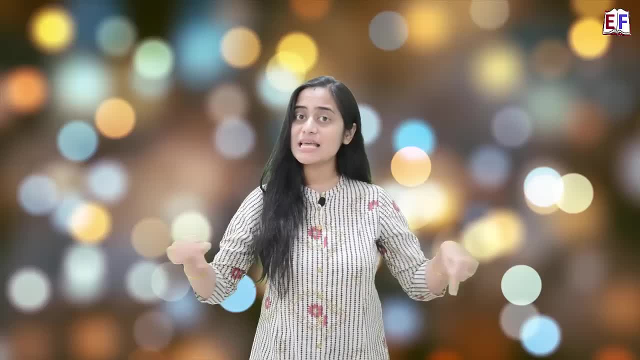 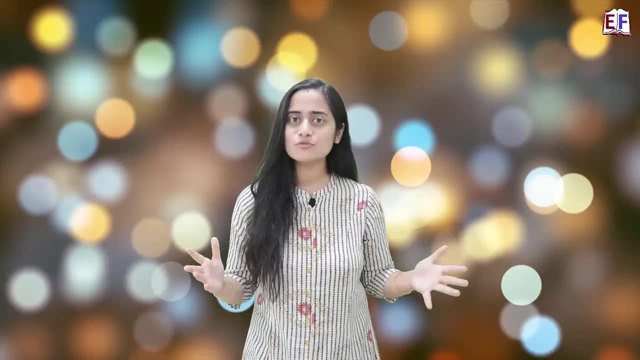 problems, please refer to the link which is given in the description section. we have created detailed video series on electric charges and fields. I hope you found this video useful. share the video. do let us know your feedback in the comment section. I'll meet you all very soon. with a new video. thank you, bye, bye.